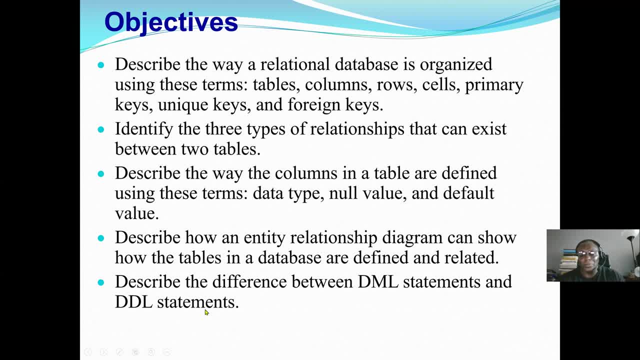 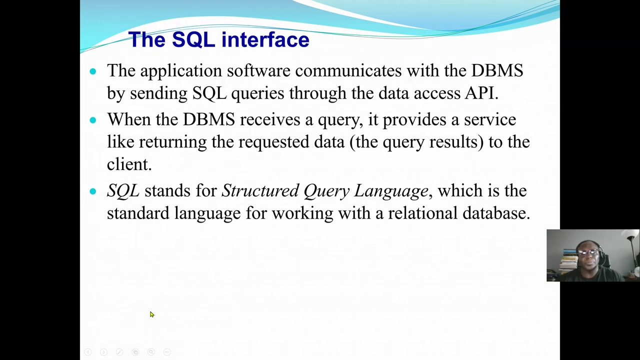 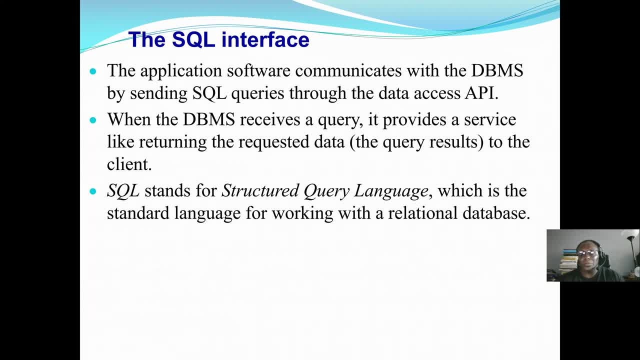 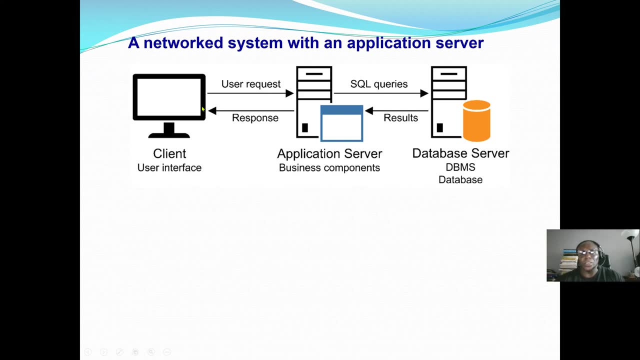 And also we're going to describe the way columns in a database are defined and related. then we may have a database server. The database server is where the database management system application is installed and also the data and information of the organization is also installed. 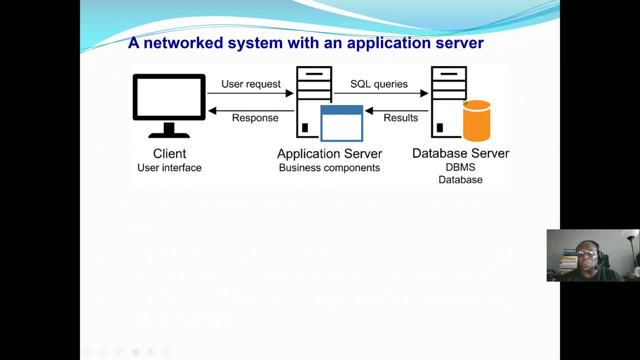 Then we may have the application server, which will interact with the database server. So when a user requests a service, it goes to the application server, Then the application server gives the SQL queries to the database server and the database server gives us results. 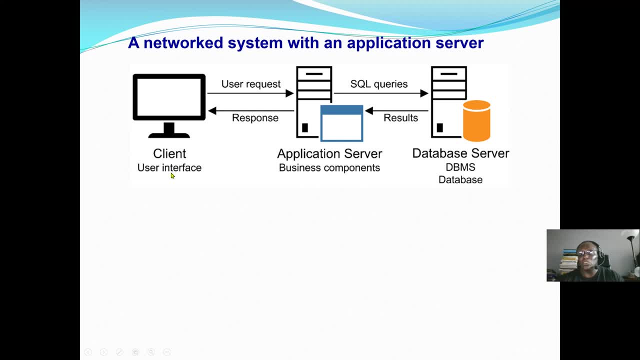 The results will go through the client user interface. So we have a user request, the direction of the arrow going to the application server, Then from there we have SQL queries to the database server. Database server gives us the results. The results will go through the application server. 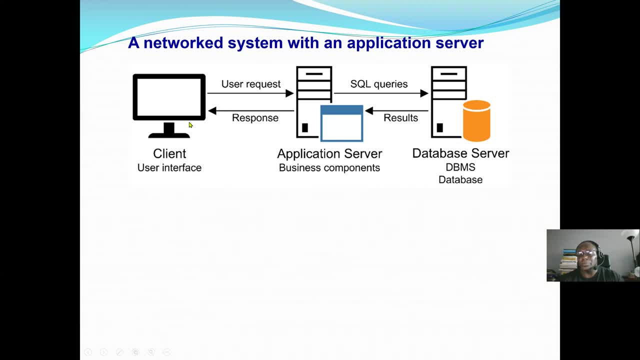 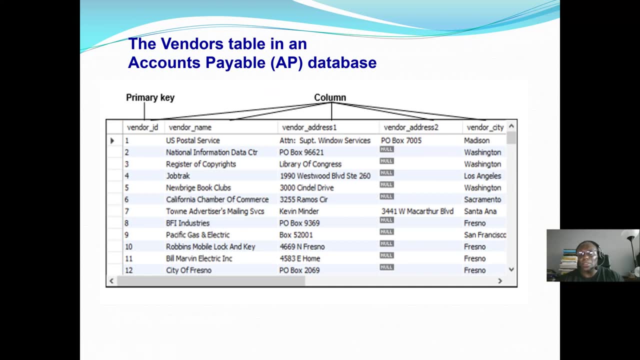 Then through the client's computer. So here in this course we are going to create a database named AP and four tables. So, example given: here we have a vendor's table in an account payable database. Again, the database name will be AP, which. 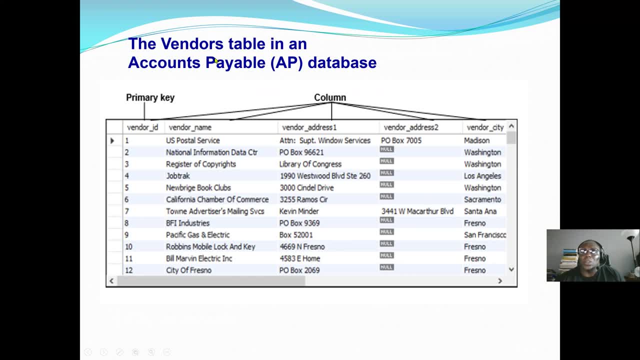 stands for account payable database. So in this, a relational database, as we said, consists of tables And we may have more than one table and there will be a relationship between the tables. So here we have a table named vendors And table normally consists of columns or the field names. 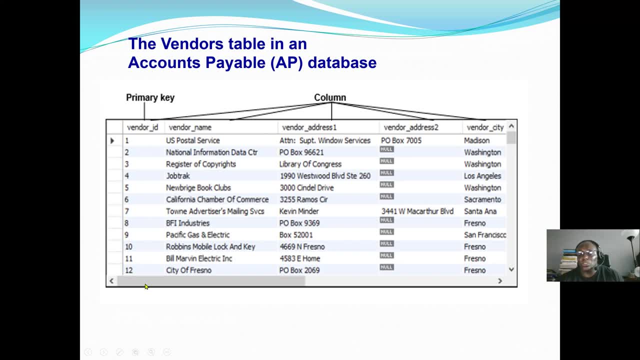 The rows will be the records. So in this case we have 12 records showing on our screen, from 1 to 12.. The column name: we have the vendor ID. We have the vendor name. vendor address 1,. vendor address 2,. 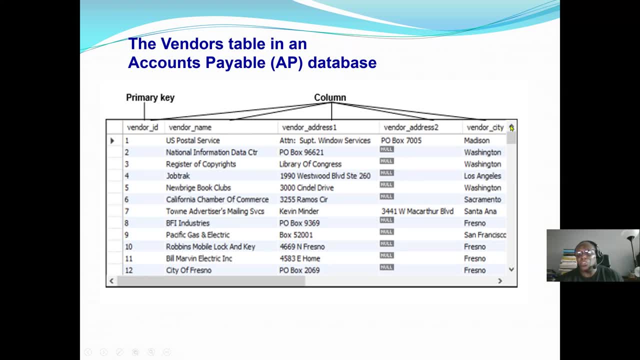 and the vendor service, And then we have the vendor ID. We may have more fields, but I think this is what we are seeing right now. Now, the primary key field would be the field that uniquely identify each record. We don't want to have a duplicate of the records. 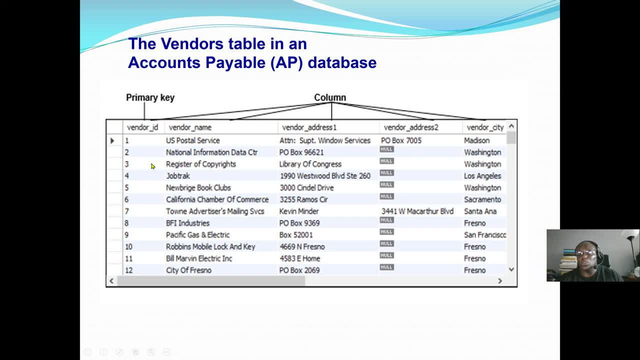 in the table. This means we are going to use more resources and also time consuming. So, for example, we know Amazon have millions of customers around the world, even employees, to hundreds or even thousands of employees. Now we don't want to enter the same customer more than once. 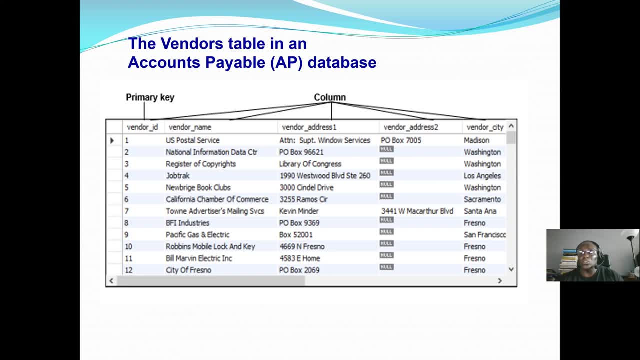 or the same employee more than once, which means we are going to waste time to enter and also the computer memory, the resources. So in a data grid system, always our table may have a special field called the primary key field that will uniquely identify each record. 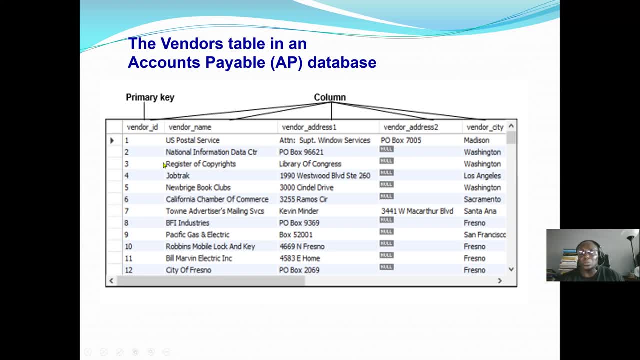 So, for example, if we have an employee table, most likely we can use employee ID as the primary key field, because two employees cannot have the same ID number. It's like a social security number. So in this vendors table we have vendor ID. 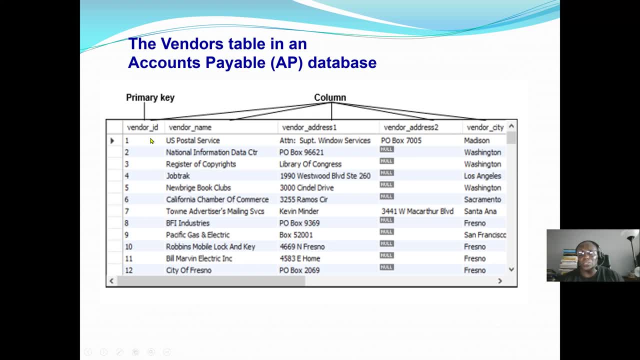 will be our primary key field and if we look at the records, we can see that the numbers are generated from 1 up to 12.. They are all unique. We can repeat the same number twice. We may discuss about primary key, forward key. 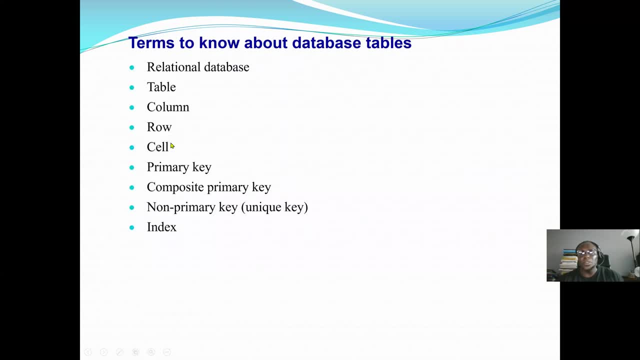 customer number again in our future lectures. so the terms we have to know in unit one or chapter one of our course is: what is a relational database? so a relational database again, is a database that normally consists of tables. a table can be called a relation and these tables have a relationship. 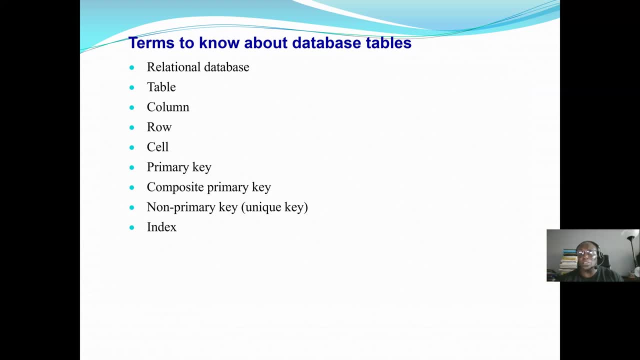 and let's say we have two or more tables and there will be a relationship between the tables. a table normally consists of rows and columns. this is the backbone of the database, where all our information will be stored. then a data base with a table may have a column. 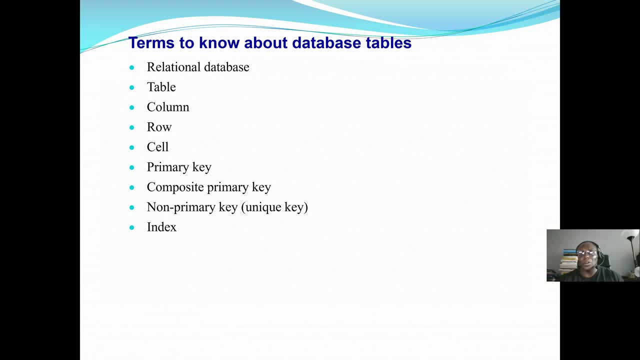 so a column will be only one field name of the. this can be a table or the entity. so for example, if we have a student table, one column name can be student name or student last name. a row will be one record. so one student, we have his last name, first name address. 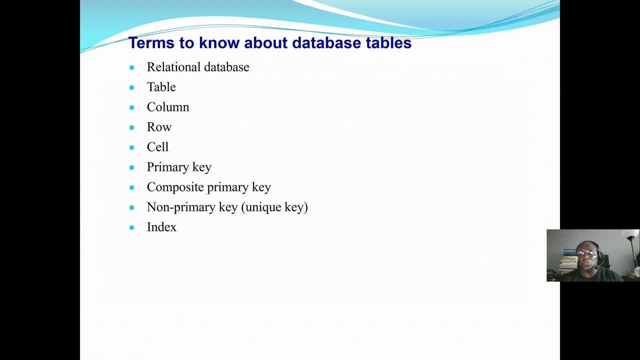 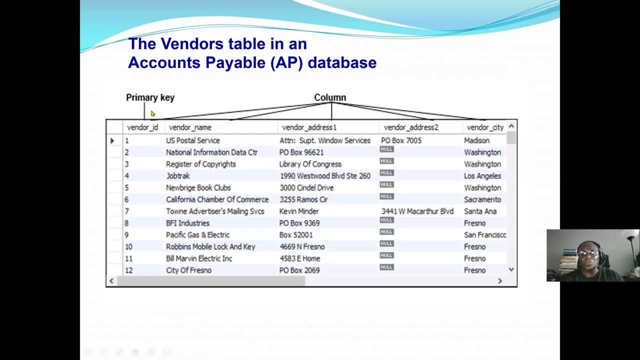 grade and all this information is one row is called a record. a cell will be the intersection of the row and column, so we'll go back to our previous example. so here we can say: we have a cell then where we have intersection of the first row and the second column is a cell which is still 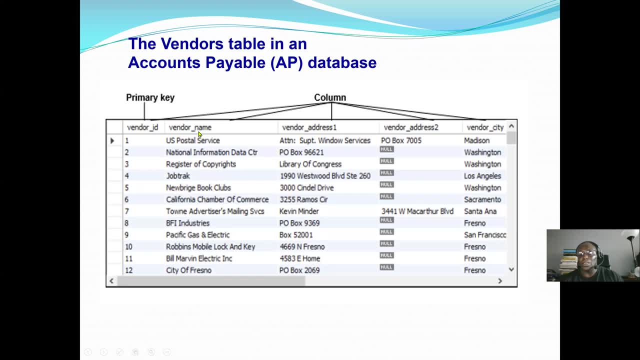 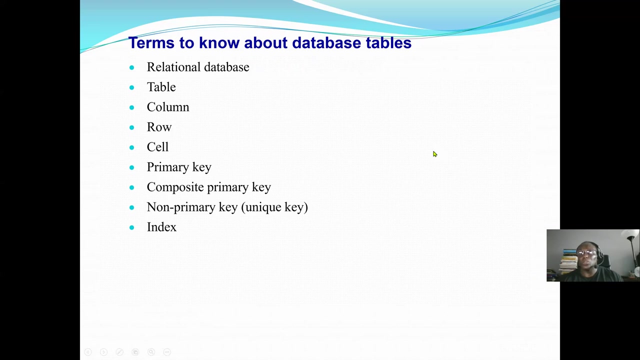 the name is us poster service. again the column name also we use the term the field name- is us poster service. the vendor id is one. so all the information in the first row is called a record or a rule which will represent one entity, for example one student or one inventory product, etc. 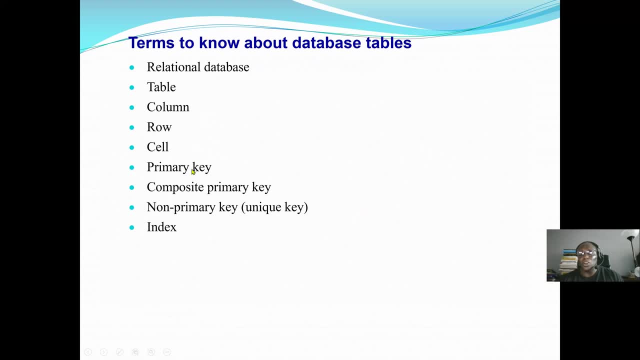 the primary key will be, as we said, a column that uniquely identify each record, a composite primary case. sometimes we may have a table whether we need at least a minimum of two or more fields in order to uniquely identify each record. so a primary key normally is one field that uniquely identify each record. when we say a 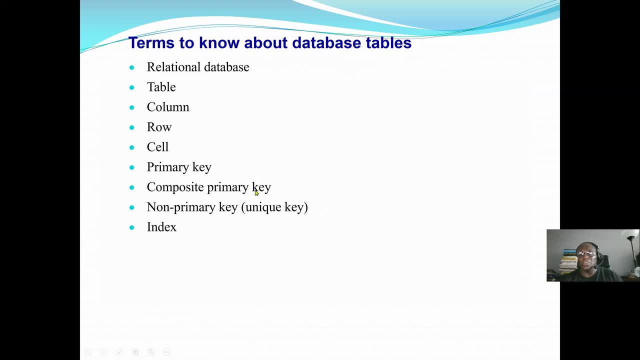 composite primary key. it means we have more than one field that uniquely identify each record. then we may have a table that has a primary key. for example, last name, first name. two students may have the same last name. two students may have the same first name. so we may have non primary key. 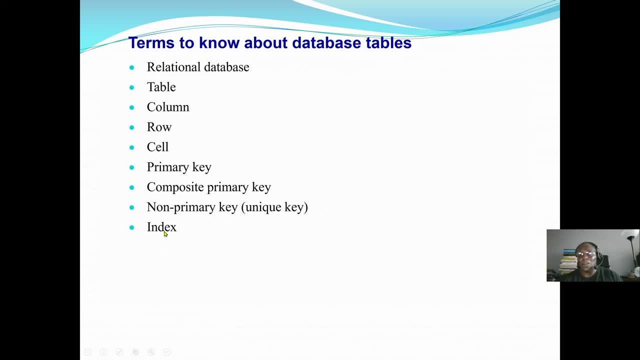 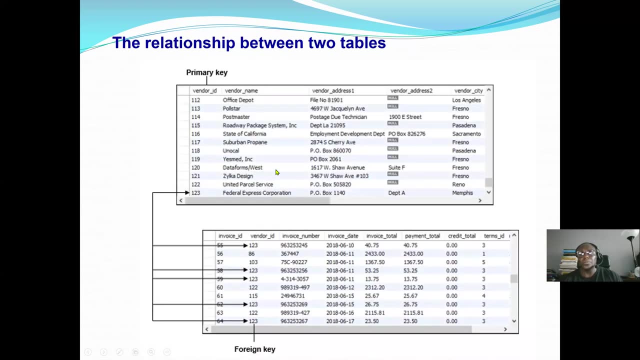 which is a unique key. then also index index allow us to access our data very quickly, efficiently. we may discuss about that also in the future. searches a relationship between two tables. You can see we have a table here. We'll call this table a vendor table. 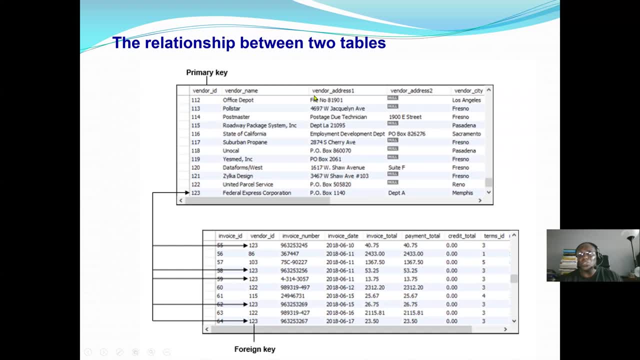 because we can see the vendor ID, vendor name, vendor address and vendor city. Then the second table. we have the column invoice ID, vendor ID, invoice number, invoice and date. So we may call the second table as invoice table. 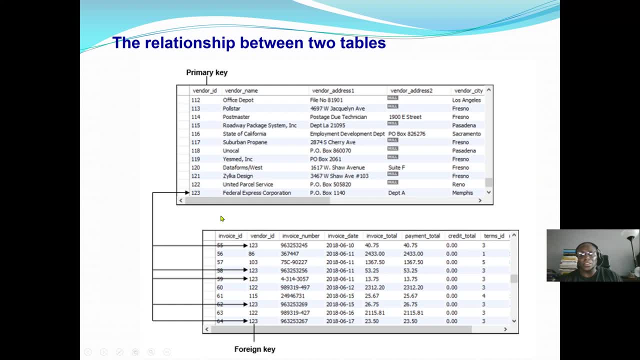 the first table as vendor table. Now, here we can see there's a relationship between the two tables. The vendor ID is a primary key field. Now, when you are creating a relationship between two tables, we always use the primary key field. 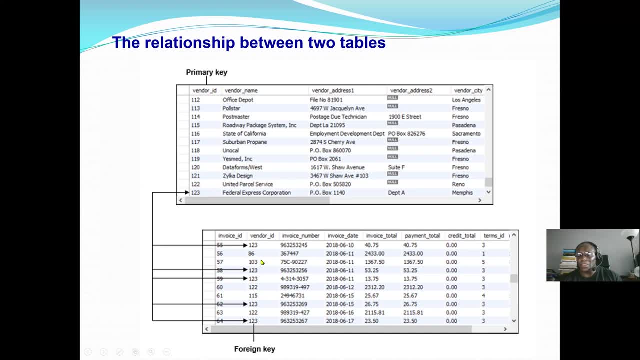 So, secondly, we also have a vendor ID in the second table, which is the invoice table, but we'll call it the foreign key. So this tells us we have one-to-many relationship. We can see that we have a vendor ID. 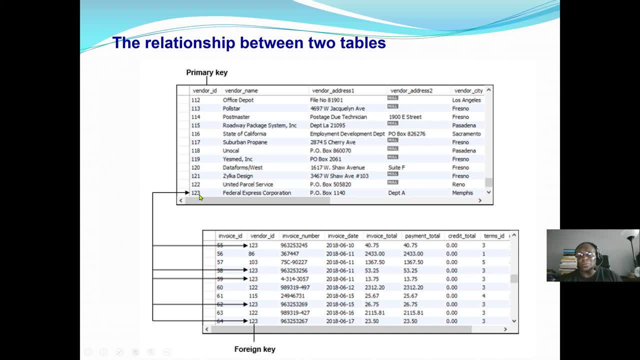 one, two, three, four, five, six, seven, eight, nine, 10,, 11 is the first one. Then we have the third table. The fourth table we call in the invoicing tab. So this one we call in the invoicing tab. 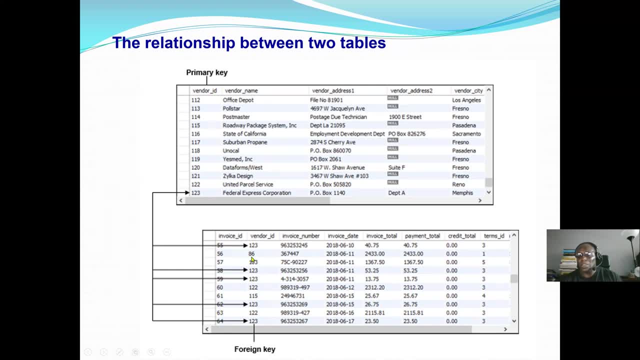 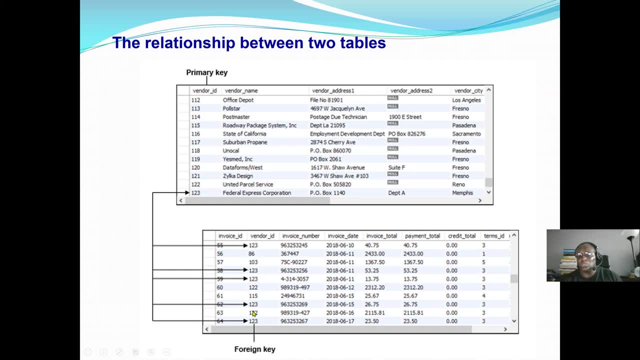 one, two, three. one, two, three. So this will tell us that we have one-to-many relationship between vendor table- again, the top table, and the invoice table, the down table. So always when we are creating relationships, 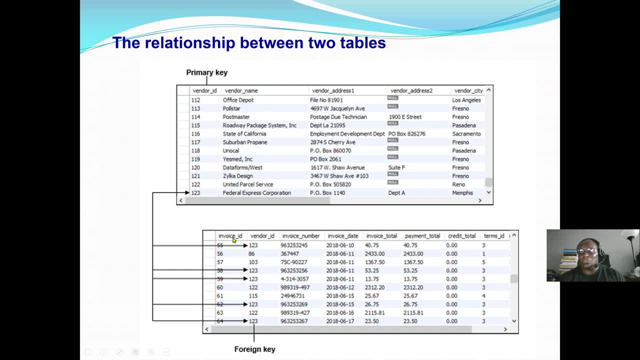 this is the first one we will call in. This will just be three, four months after this one. between two fields, we always use the primary key field, So vendor ID is a primary key field in vendors table. So it appears only once. 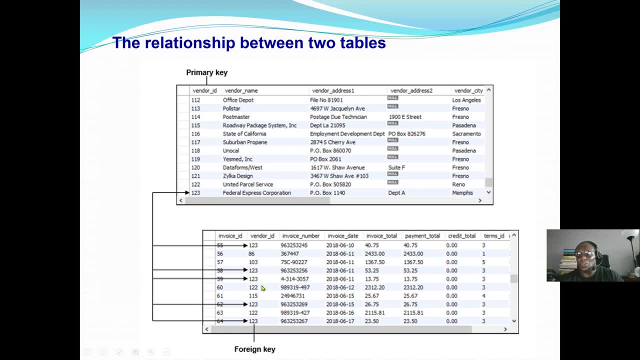 but vendor ID field is a foreign key or secondary key. Sometimes we use the term secondary key or foreign key in invoice table And we may discuss this more detail and we may write a SQL command that make it possible. So the terms we should know about table relationship: 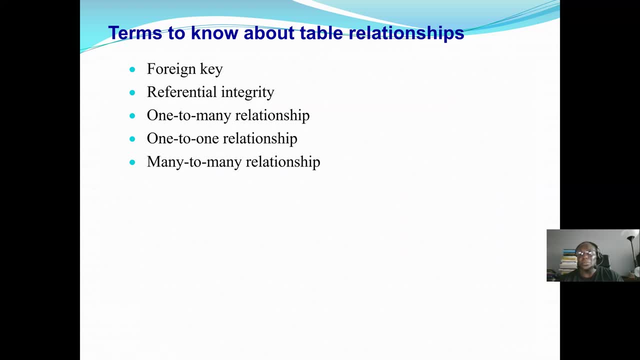 will be the foreign key. as we said, the foreign key allow us to create a relationship between two tables And the foreign key is a primary key in another table. Now, when we are creating a relationship between two tables, we want to make sure. 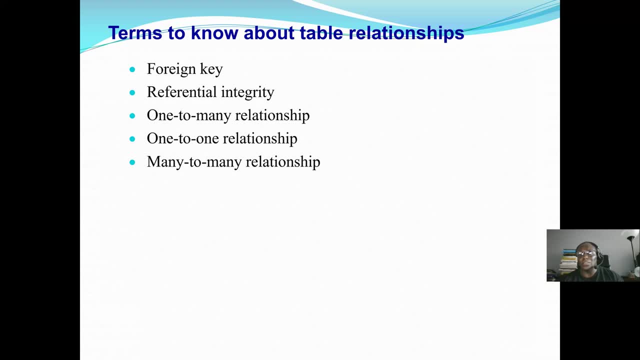 there's no any errors data in terms of if I updated or delete or enter new information in the first table, it should be updated in the second table, in the table that you have a relationship with. So here we have to enforce what we call. 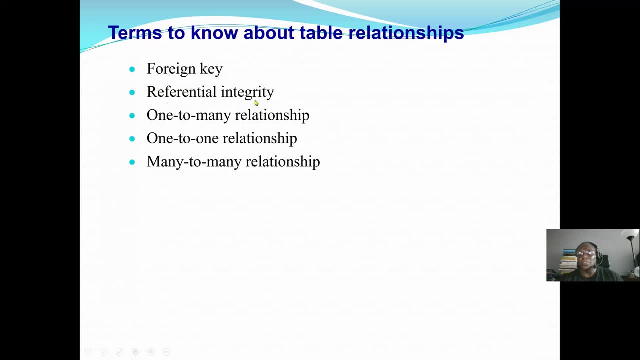 the referential integrity to make sure again data will be consistent and no error. We also have one to many relationship means, as we said earlier, one table may have only unique field. Then the second table that you have relationship can have many fields. 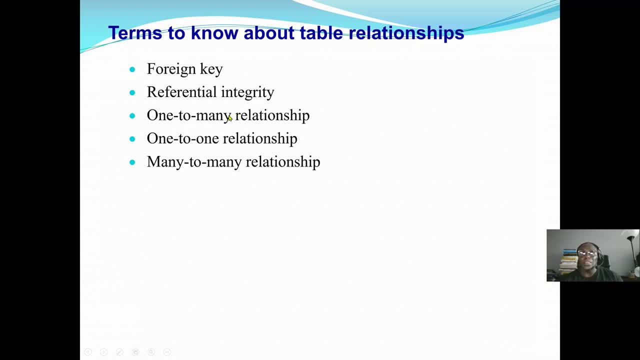 So one to many means. again, we have a vendor ID. can be entered only once in the vendor table, but it can enter as many as we want in the invoice table. So we have one to many relationship. Sometimes also we have one to one relationship. 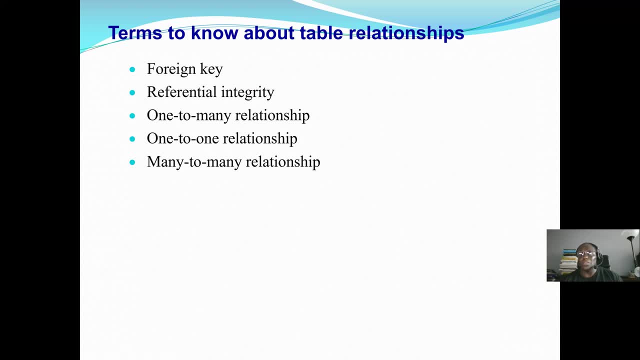 which means both relationship. that field should be unique And we may have many to many relationship also. So these are the three major relationships among tables in a database system: One to many, one to one, many to many. We may discuss this more detail later on. 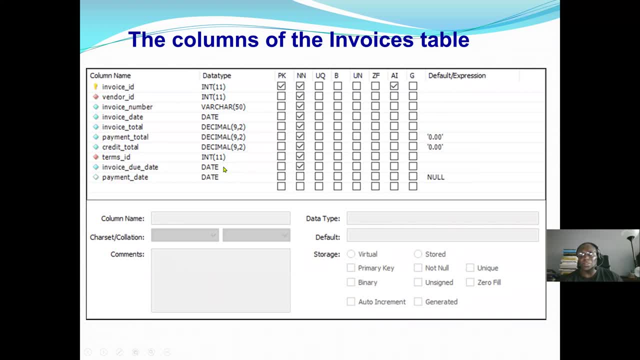 So in this course we are going to use MySQL And in this screen we are seeing here- this is the screenshot of the workbench. So here we create the columns of the invoice table. So first column name is invoice ID. We have vendor ID. 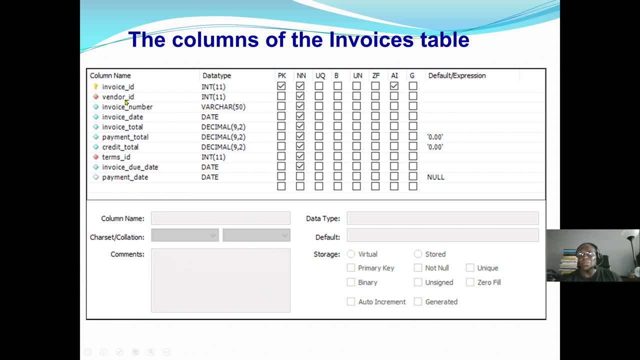 Vendor ID will be the, the foreign key, because it's a primary key in vendor table. So anytime we create a field we may have the field name or the column name. Then also we have to add the data type. The data type will tell us what type of data we can store. 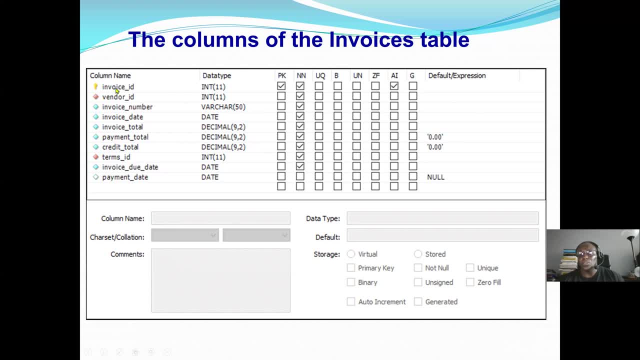 in that column name or in that field. So for example in invoice ID the data type is int, which means we can put digits, And they have 11 here, which means we can go up to 11 digits. Then we have PK stand for primary key. 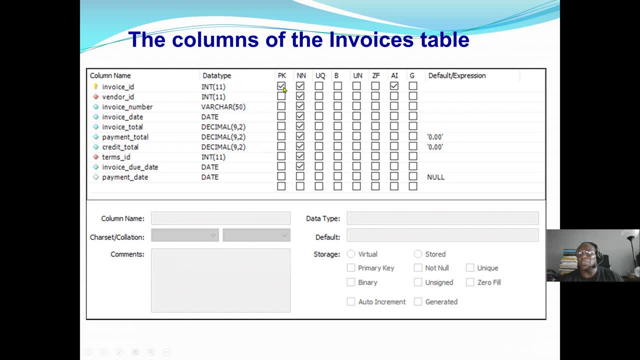 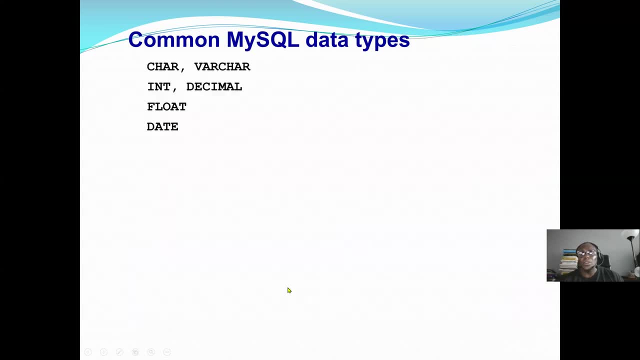 So the invoice ID, we are going to identify it as a primary key field And again, we may discuss this in the future lab work. Also, when we have a field, as we said, there's a data type. We are using MySQL in this course. 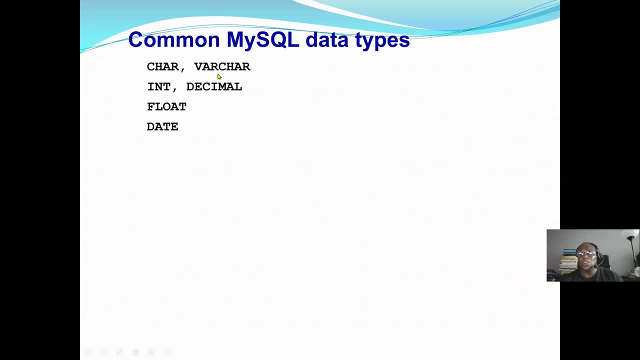 So MySQL data types can be char, which is character, or varchar, many characters We can have. int means a whole number, Decimal means a decimal number. Same thing apply to float, also means a decimal number. Now the difference between decimal and float. 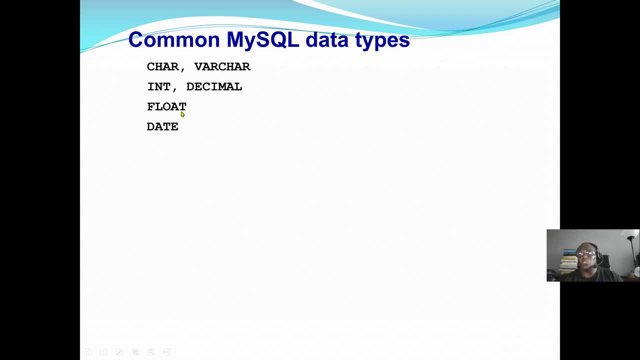 is the number of decimal places which we call the precisions. It depends. And also we have a data type for date. if we are storing date in a specific column. Now, in terms to know about columns, we should know the data type. 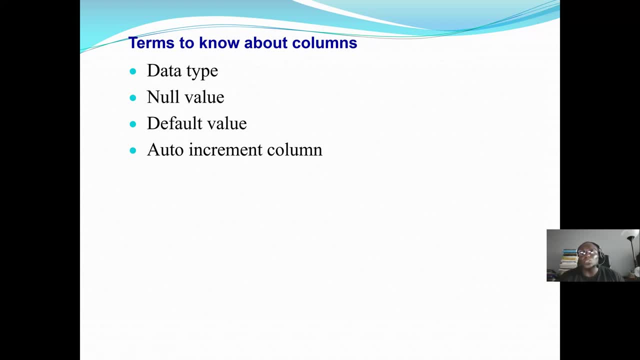 to get a data type, represent the type of data we can store in that column And we saw, example, a character or a test or a whole number which is int, or a decimal number or a date, A new value means in that very column. 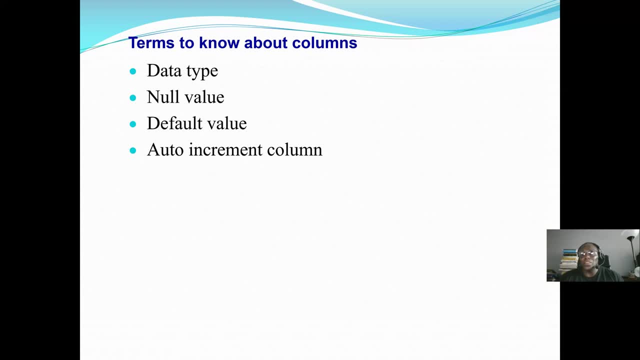 we can leave it empty. A new value means there's nothing, even if we have a, let's say, a column named balance, balance account And we put zero, Zero is a value. But a new value means we don't put nothing, it's empty. 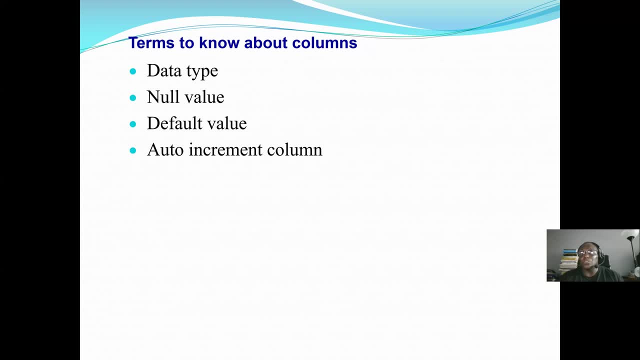 So normally when we have a unique field, like a primary key field, we always specify that not null is not allow, Null is not allow. So always we say: not null, We will select not null, so that because that is a primary key field, 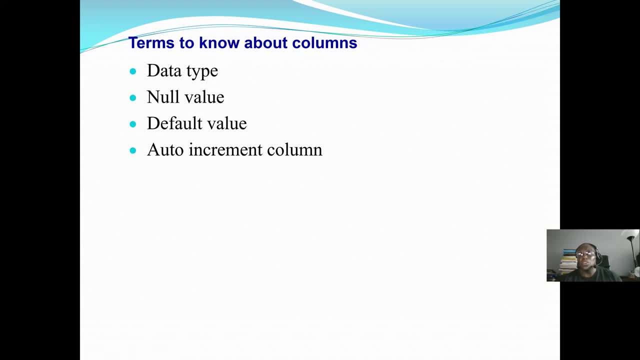 we can put zero. So primary key field is a field that uniquely valid for each record. So if we left it with nothing then it cannot do its work. So primary key field always should be not null. Default value means anytime we enter a record. 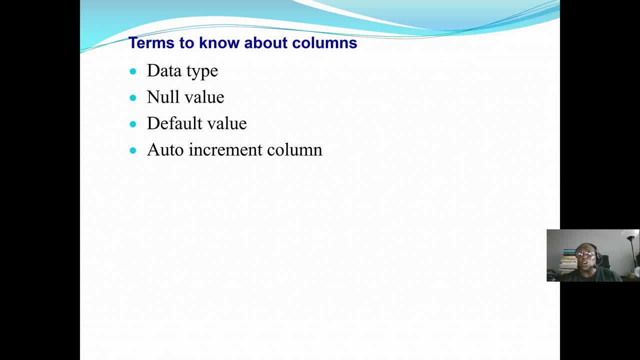 a special default value will appear. For example, I know all my customers are from New York. New York State is NY, abbreviation of NY. So in the state field instead of always typing NY, NY, I can have a default value for state field as NY. 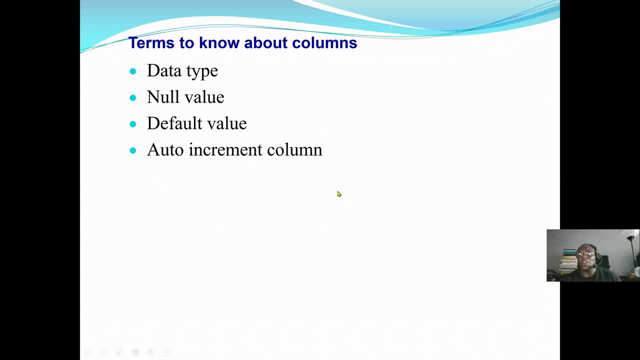 So when I start to enter a record, the NY will come by itself. I don't need to type it. Also, when we have the primary key field, if we don't want to generate the numbers, we can use what we call the auto. 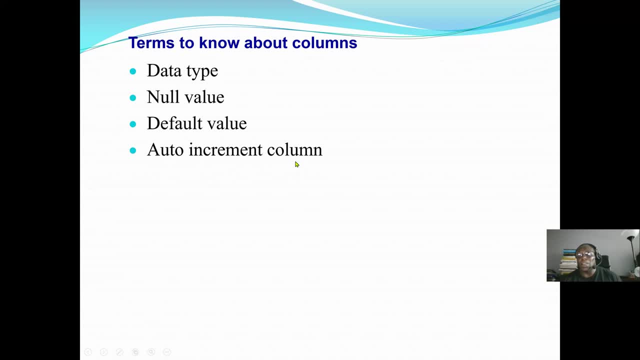 or automatic increment column, which means when I enter the first value or the first record, the number will be one, Start from one. Second will be two, three, four, going So auto increment. Now, when you select a data type as an auto increment, 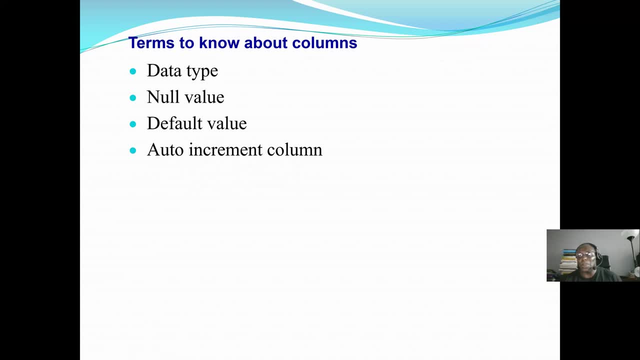 you can specify: you don't have to start from zero or one By default, start from one. You can specify that, okay, I want to start from 10,000, or I want to start from 500.. And also you can specify that you want increment of five. 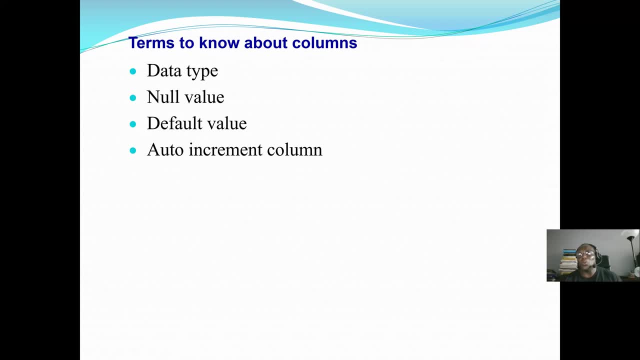 instead of from 1,000 to 1,001, I want from 1,000 to 1,000.. 1,005, et cetera. So auto increment. column again is a data type. Normally it's a whole number increment. 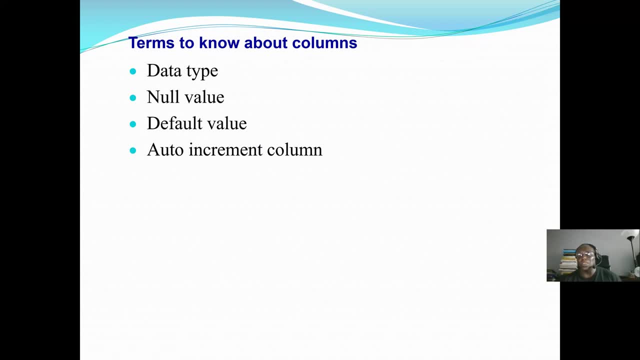 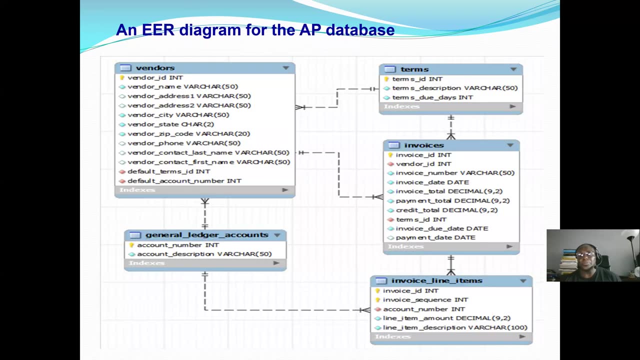 but how you specify. By default it's to start from one to increment by one, But you can start from any number and you can increment by any number. So this is what we're going to do in the lab work, And this is again chapter one of the course textbook. 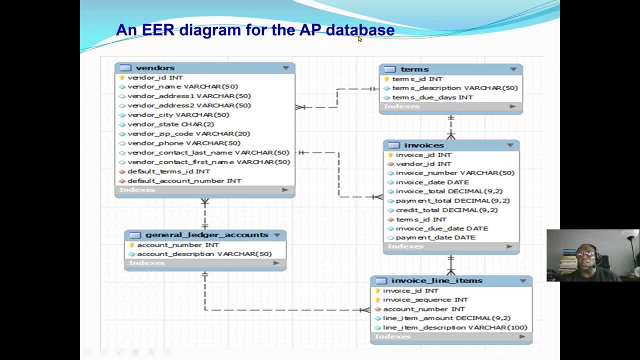 So the first thing we're going to do we are going to create our account pair with database. When we create our account pair with database, we are going to use it throughout the course. We're going to write a lot of select statement indices. 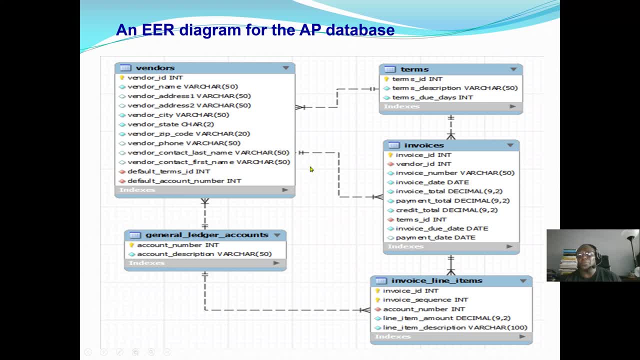 We're going to create a views, queries, everything. So this is how the database will look like. It will have five tables. The first table is vendors. We can see vendors have a relationship with a second table, named terms. We also have a relationship with another table, named invoices. 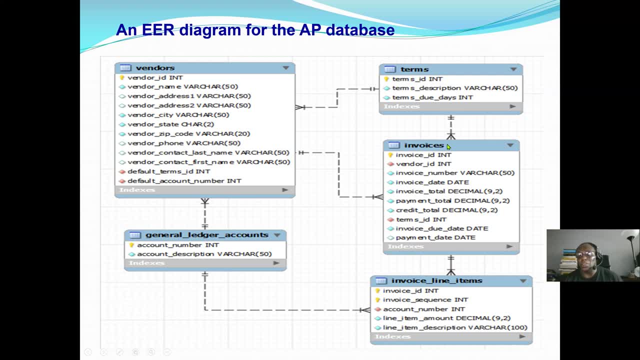 Invoices have a relationship with the terms table, which is one to many, And also invoice have a relationship with vendors, which is also one to many relationship. Then we also have invoice line items, which have a relationship with invoice table also. So again, we will go through in chapter two. 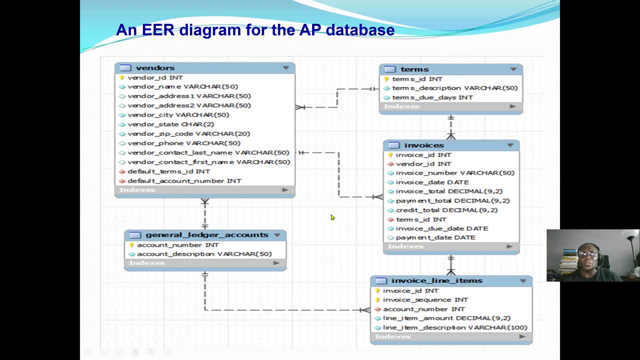 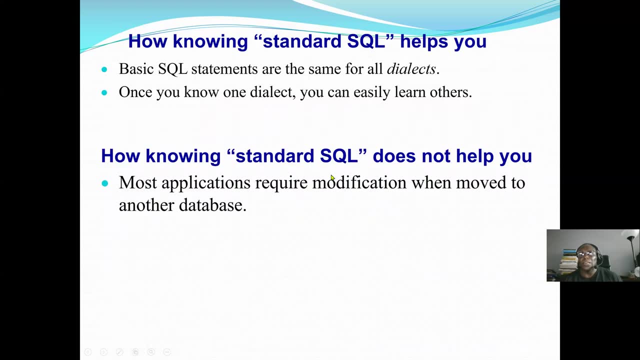 we will go through all the scripts, the command, the SQL command to create all these tables in the database also. So knowing how a standard SQL can help us, see how knowing standard SQL helps you. We say basic SQL statements are the same for all dialects. 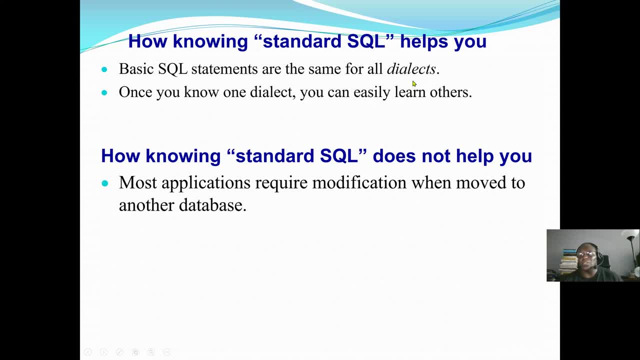 And what we mean by all dialects is that database system. we have different vendors, for example, Sybase, Microsoft, Oracle, et cetera, or MySQL, which is the one we are using for this course, And the standard SQL script. 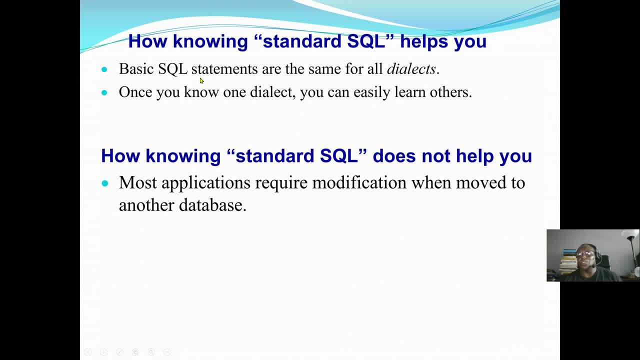 we can use it for most every different types of database vendors. So once you know one, for example, once you know how to write SQL for MySQL database or for Access or Oracle, it's easy to learn the rest because, again, SQL is a standard language for. 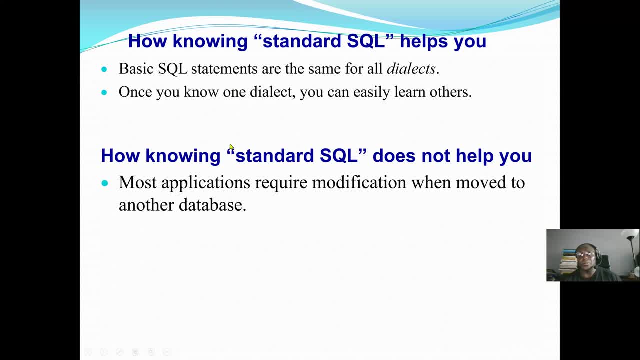 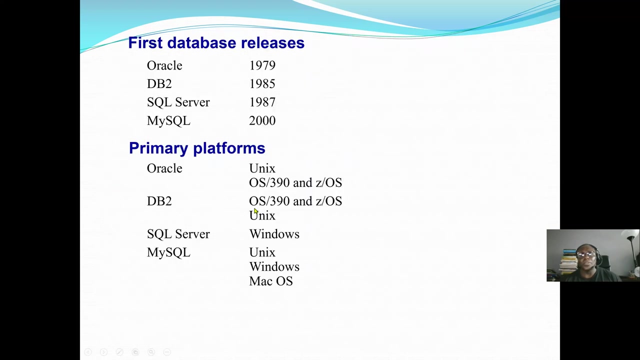 database system. Also how knowing standard SQL does not help you. We say most applications require modification when moved to another database. For example, sometimes we have some data types in Oracle which is not in MySQL. Still we can say SQL is a standard language. but sometimes we may have a little bit differences like data types more or less in different vendors. 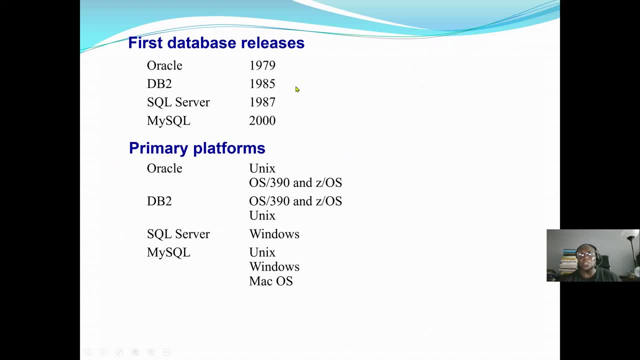 So this is our first database release was Oracle 1979. And when we say a database, we mean a relational database release Before 1979, we have files that are normally stored like a test file, Not a relational database system, but we still have a storage system by some relational database. 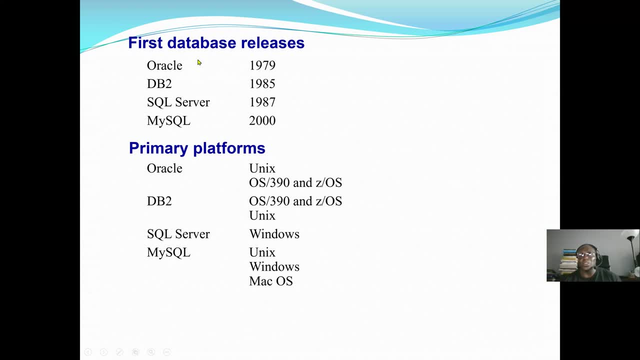 The first relational database system, which we call the database management system, was released by Oracle 1979. Then IBM released DB2, which is database 2, in 1985. Then Microsoft released SQL Server 1987. Then MySQL. MySQL again is a free open source. 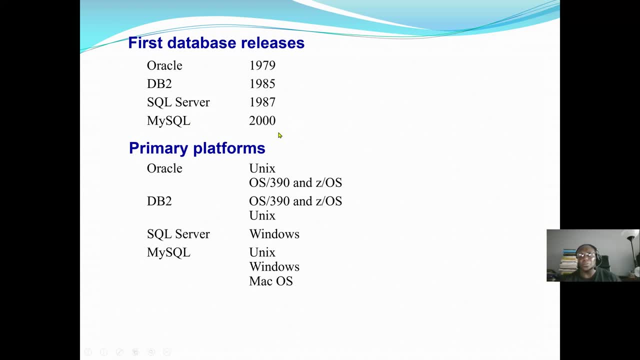 The database system was released 2000.. Now the primary platforms for Oracle. Oracle database can be used in Unix operating system or OS 390. ZOS, Also the same to the database tool by IBM, can be used in Unix and also OS 390. 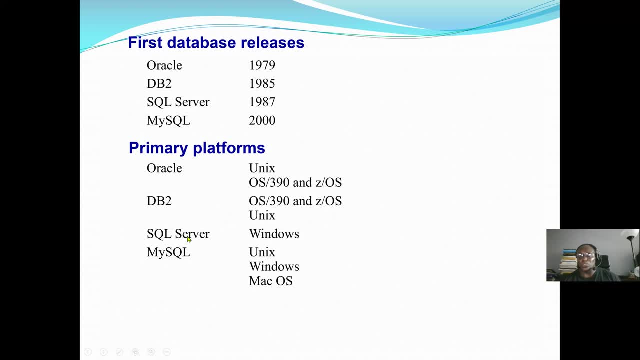 But SQL Server, again from Microsoft Corporation. So it runs on Windows. MySQL is the best. It runs on the three major platforms: Unix, Windows and also Mac OS. Again, MySQL is a free, open source. Oracle belongs to a company. 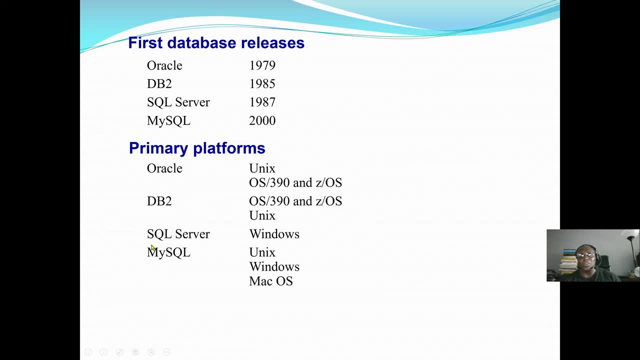 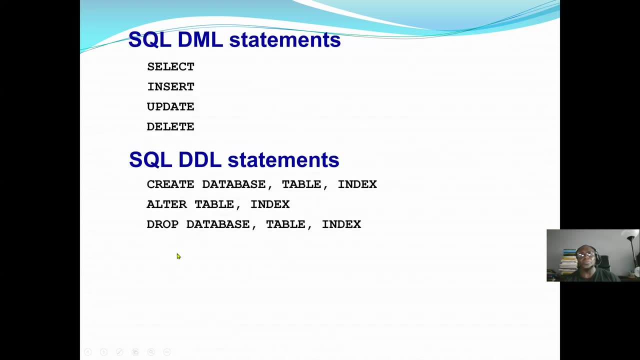 It's not free. DB2 also for IBM, company SQL for Microsoft, But MySQL again is an open source, Free. Now with the SQL we have the DML statement, which is the data manipulation language, For example. we will go through how to write the statement for select, insert, update and delete. 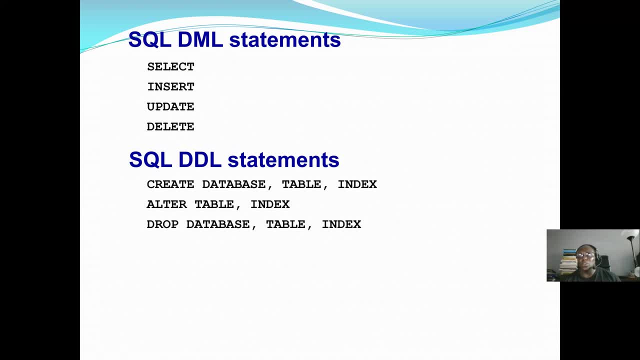 Select is for query. I have a database with students And students have different types of grade from A, B, C, D and F. So I'm going to write select statement to only see the students that get only A grade or that have only B grade. 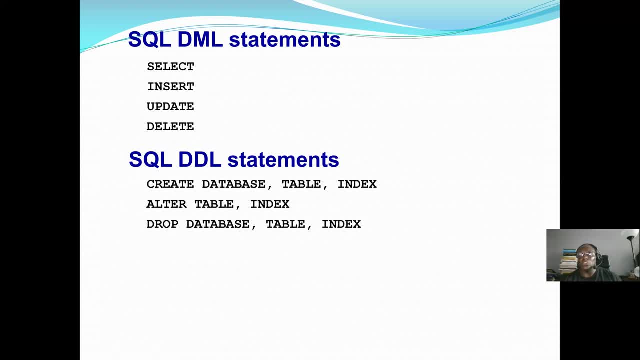 So I will use select Now. if I want to add a new record to my table, I will use the insert command Now. if I want to change any value of my records, I can use the update. Update normally goes with the set command. 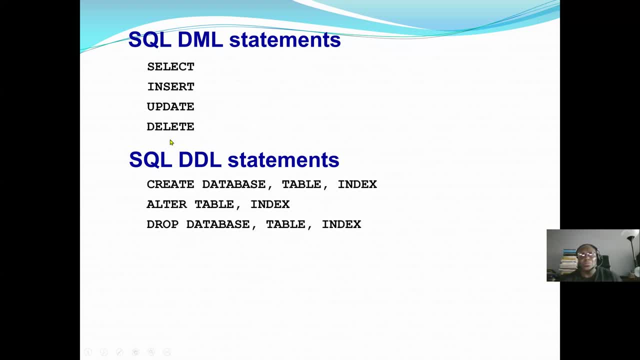 So then if I want to delete Any item, I can use delete. We can see that delete means we are going to delete a record But not the whole database or the whole table in the object. Now if I want to delete a database or object, I will use the command drop. 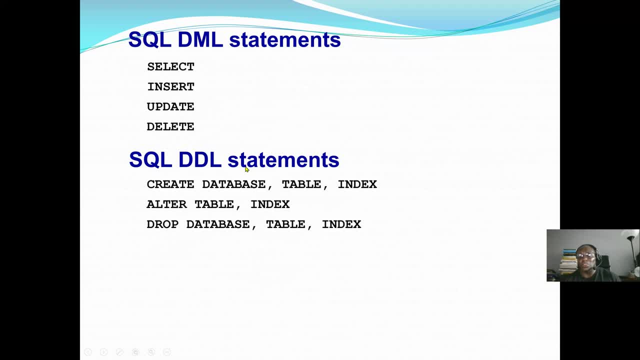 Drop normally belongs to data definition language, DDS statements. So with the DDS statement we can now create the database object, Such as table index, view etc. And also we can delete. We can delete it. We can also alter the table. 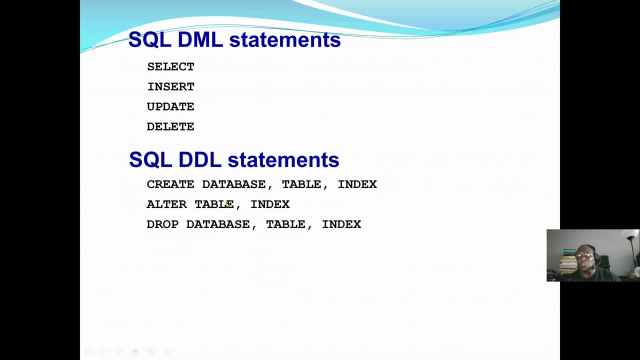 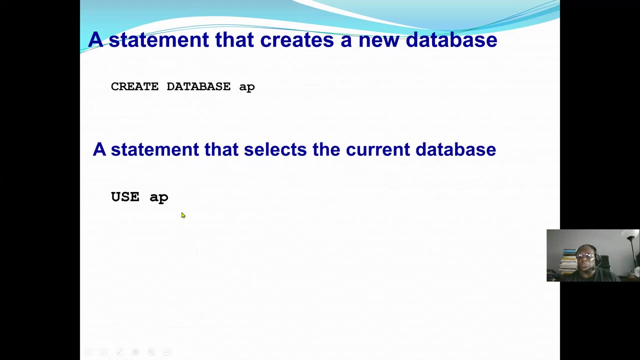 Alter the table. example will be: I'm adding a new foreign key, Or I'm adding a new primary key, Or I'm deleting some record or deleting some columns. So we'll go through some of the few statements here, But in chapter two we may go into detail. 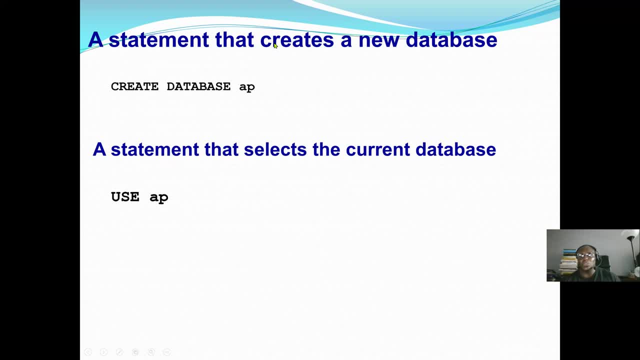 So first we start with the statement that executes, And when this statement executes we are going to create a new database. So the command to create a new database in SQL is create database. So create database. AP will be the database name. So I will start with the command create database. 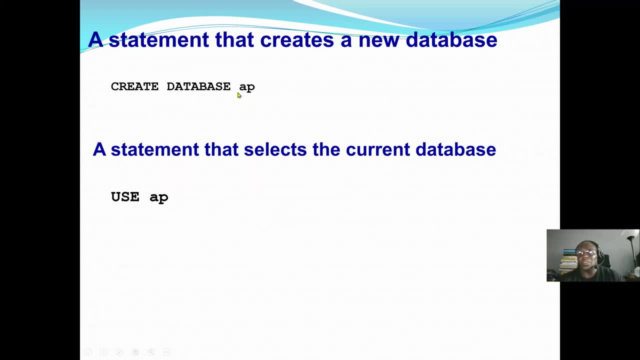 Then the database name. In this case I'm creating a database name AP. Now if I have the database and I want to use it, I can either use my mouse to select the database in my workbench on the navigation area, Or I can use the command use. 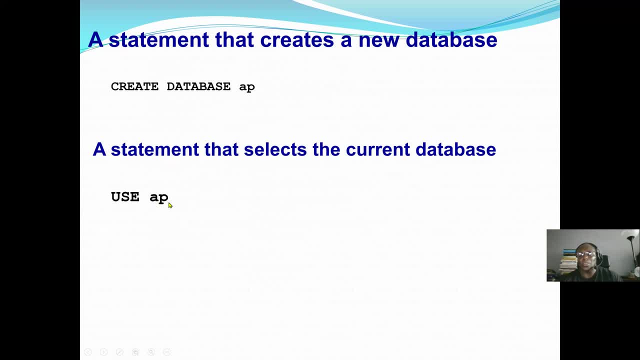 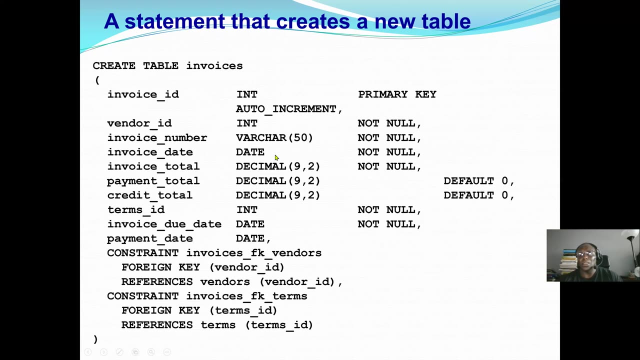 So when I type the command use AP and I run it, AP database will be selected or will be ready to be used. So this example to create a new table. So, as we said earlier, we are creating a database name AP, Then we are going to create around four or five tables. 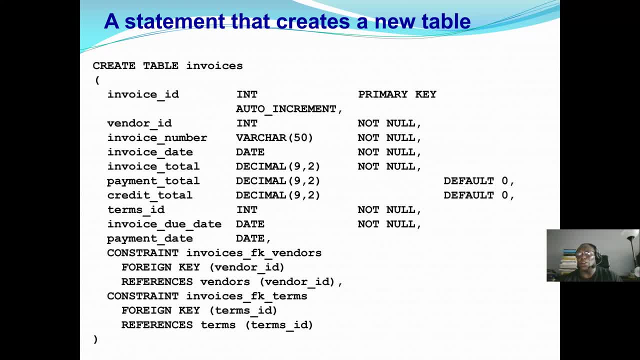 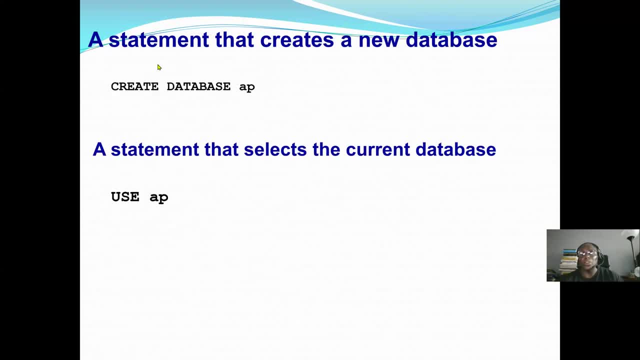 This is the database we are going to use throughout the course, The lab work. So we have our database. So first thing we did, we create our database name AP. Now, when you create a database, you want to use it because we want to create a table. 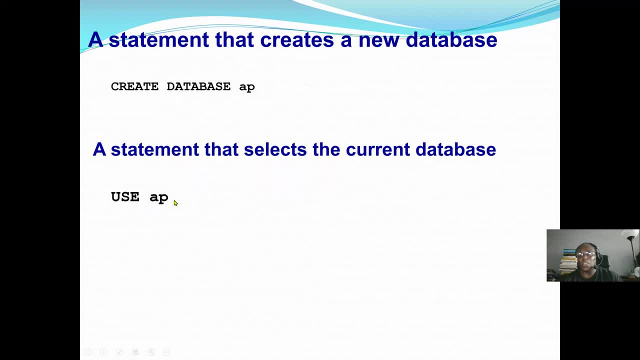 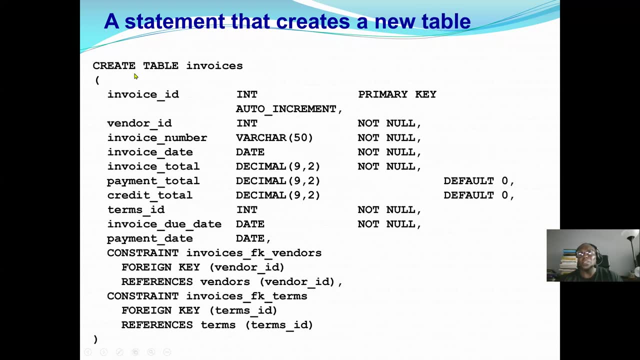 So we'll run the command use AP Or you can use your cursor to select the database. Then first we create a table. So, creating a table, we use the command create table, Then the table name. So in this case we are creating a table name. invoices. 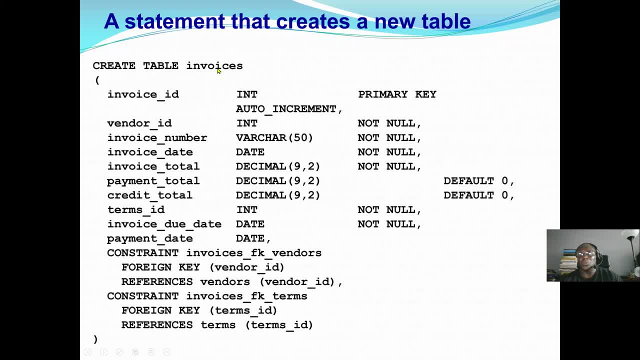 So create table invoices And the table normally consists of columns. So we have the column names: Invoice ID, Vendor ID. Invoice number, Invoice date. Invoice total Payment, total Credit, total Terms ID. Now, when we look at the second column, those are the data type for each column name. 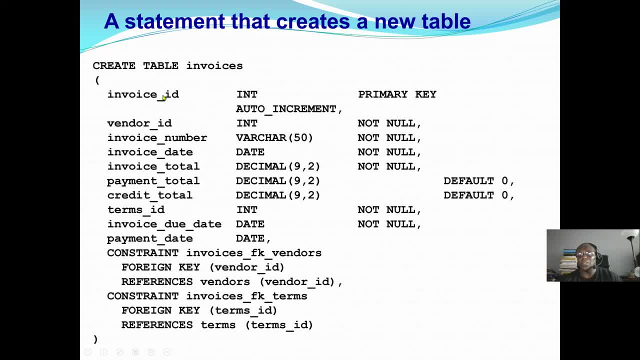 So, for example, I have invoice ID, The data type is int, Which means I can put only O numbers. I can have only O numbers there, And also invoice ID is a primary key field. So we have primary key. As we said earlier, primary key field is uniquely identify each record. 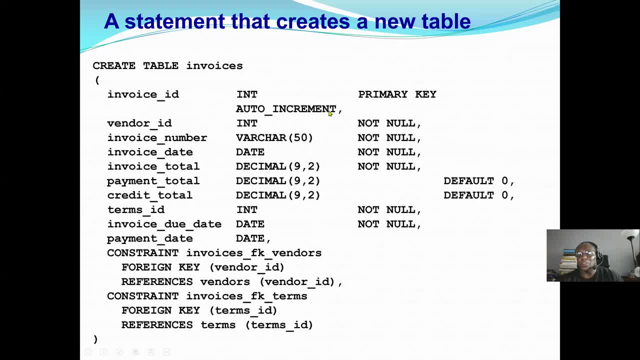 And the primary key field: we make it auto increment. Here you can see that we have only auto increment, Which means by default we are starting from one And we're going to increment by only one. So we start with one, two, three, fourth record, fifth record, etc. 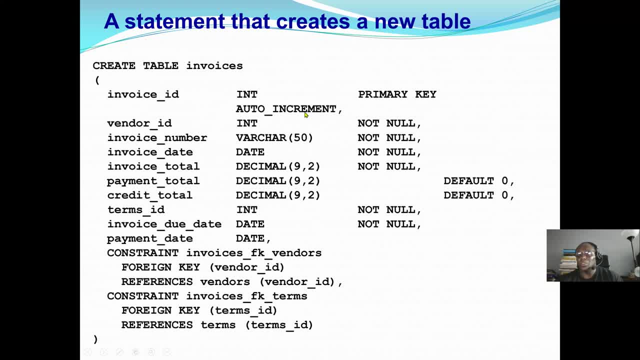 Now I can also create auto increment field. Then I can specify: okay, I start from 10,000.. And I'll increment by two, So 10,000, 10,000, two, 10,000, four, etc. 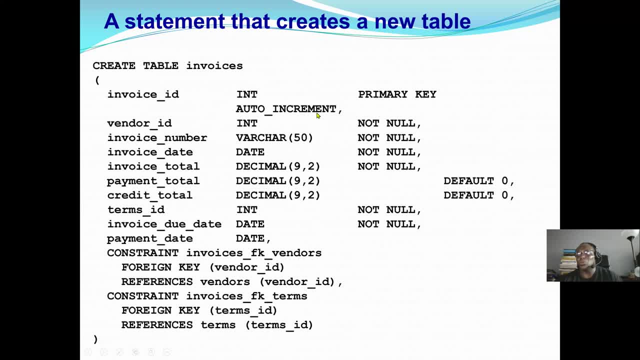 But we need to specify Here. we just said auto increment, So we start from one, two, three, four. Also, we can see the vendor ID is int. We want to make sure that the vendor ID, the user, don't leave that field empty. 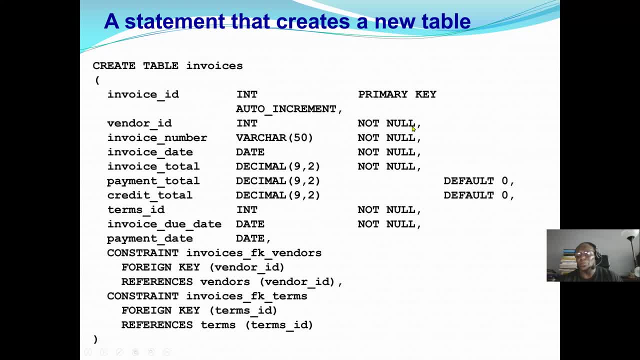 You must enter a field, So we'll make sure it's not null. Not null means you must have something there, Even if it's zero. write a zero instead of leaving it with nothing. Primary key automatically also is not null. We always have to have something. 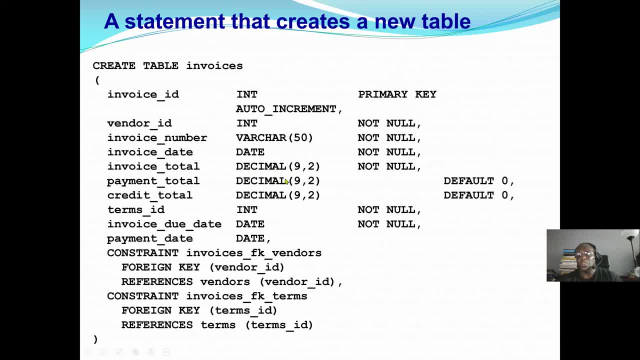 So, for example, here we have decimal nine. two. This means we can enter a decimal value for invoice total, And nine means we can have up to nine digits. Two means we can have only two decimal places. So this should be like a dollar, maybe $20,, 50 cents. 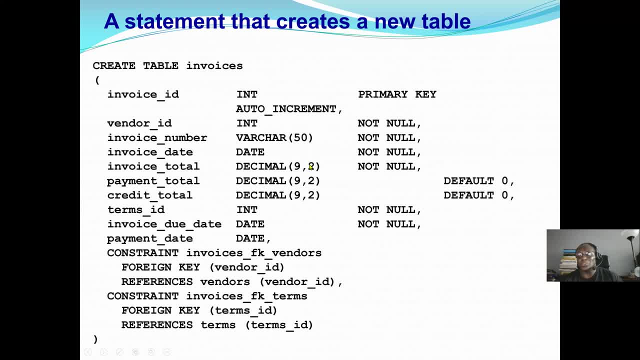 Always the cent will be two decimal places. So again, those are all the fields. We will go through all these fields. But again, as we said, int is the whole number. Auto increment: the computer will start from. We didn't specify where to start and how to increment. 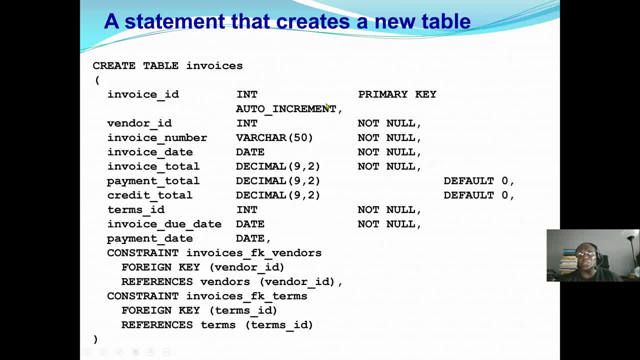 So it will start from one. increment by one, which means one, two, three, etc. Varchar means we have more than one character. here We can have up to 50 characters for the invoice number. Data type, date means we can enter the date in that field. 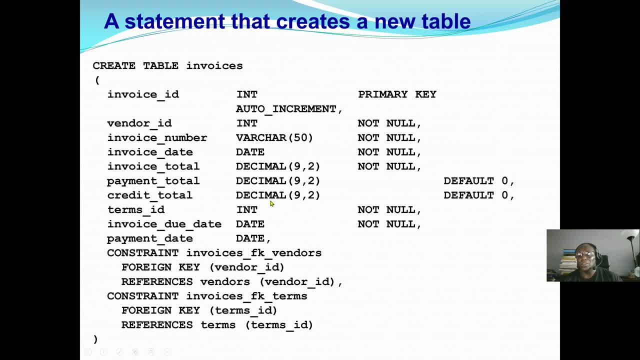 Then the last three. here we have decimal, which means decimal value with up to nine digits, And then two decimal places. So nine is the number of digits. The second value, two, means the number of decimal places, And we also have invoice due date. 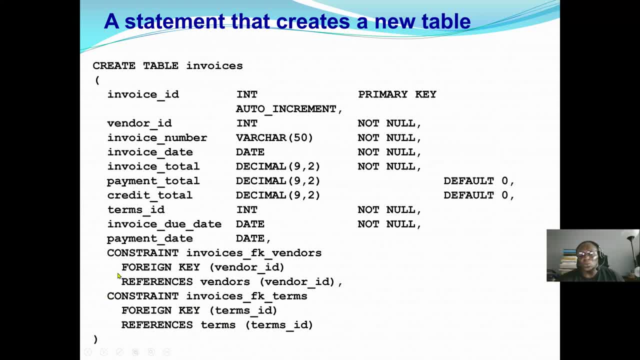 Then here we are creating a foreign key. So we use the command constrict. The foreign key name is called invoices- FK vendors And we have the command foreign key. But the foreign key will take an argument of the name of the field. So here we want to make invoice in the invoice table. 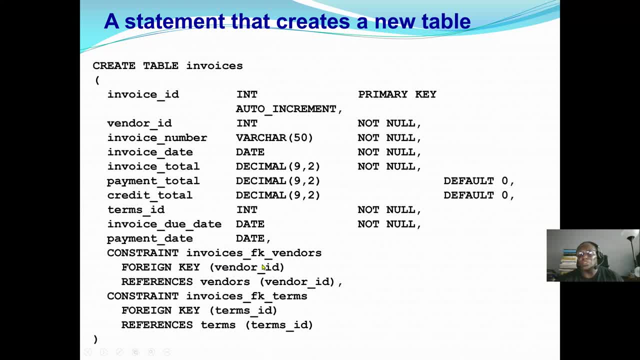 We want to have the vendor ID as a foreign key. You can see that we already, in order to say we have the vendor ID as a foreign key, we should have vendor ID already in the column name, So we can see. our second column is vendor ID. 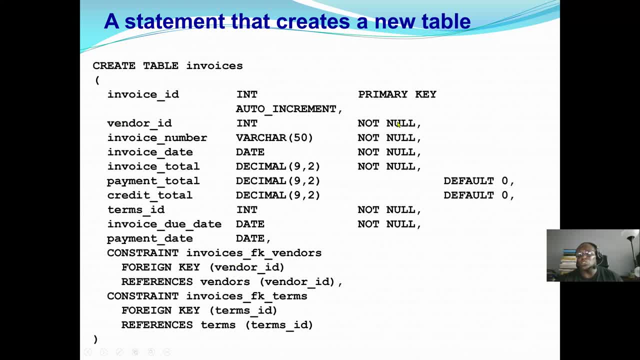 Because it's going to be a foreign key. that's why we have not known. So again, the command is constrict. Then the name of the foreign key Invoice: FK vendors. Again, name can be any name you choose, But we have to use the command constrict and foreign key. 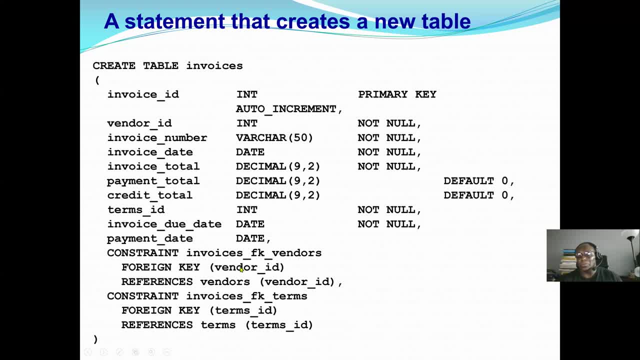 After foreign key the argument will be the field name, The column name or the field name that you want to make as a foreign key. Here we are making vendor ID. Vendor ID must be already listed here as a field. So our second column name is vendor ID. 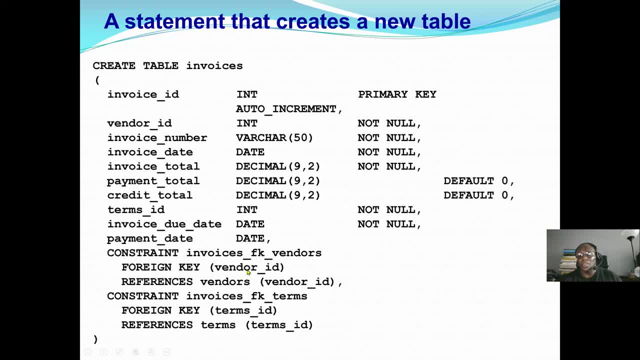 We are making it as a foreign key And this will be referenced. So foreign key makers create a relationship between two tables. So we use the command references to the vendors table And the vendors table. we are using the vendor ID also, So vendor ID is the primary key field in vendors table. 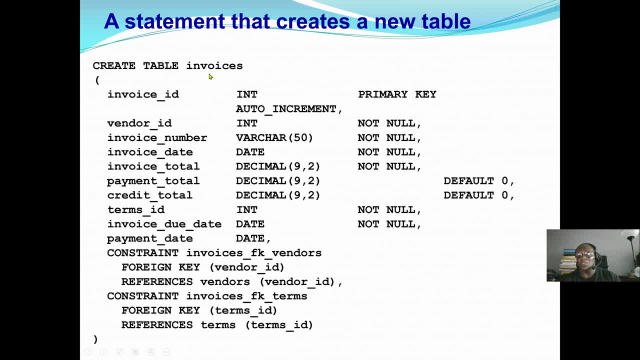 And vendor ID is a foreign key in the invoices table, So we are using it to create a relationship now. So here we have a relationship. So here we have a relationship between, again, an invoice table and vendors table, Using the vendor ID field to create the relationship. 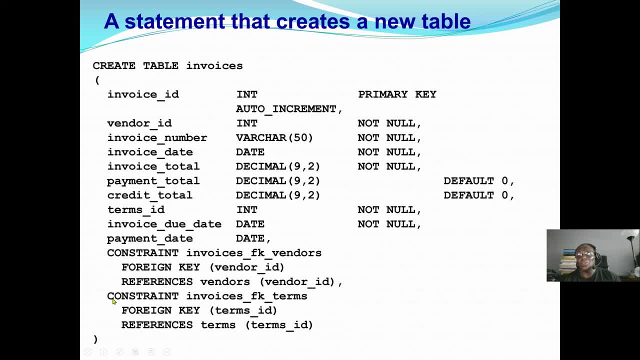 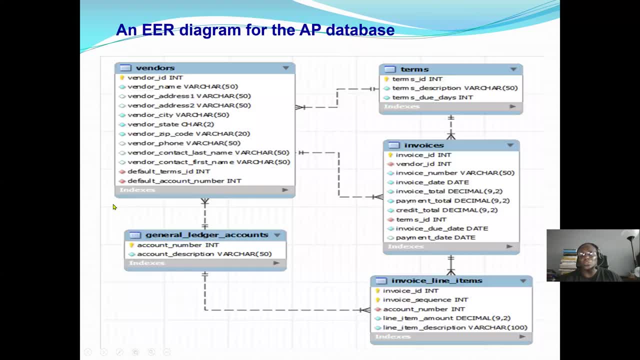 Secondly, we have another relationship. here Again, the table can have as many relationships. It depends on the design. So let's go back to the database before. So, for example, if we look at generated ledger account, We have two relationships. 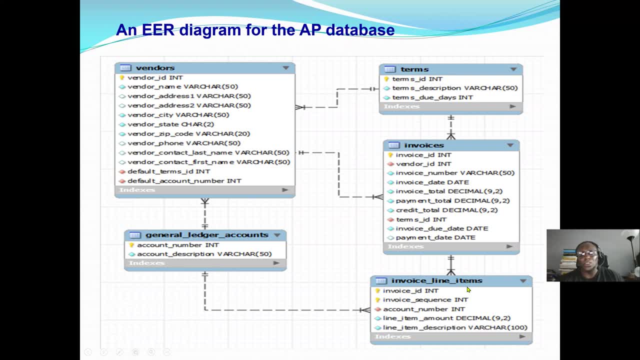 We have a relationship between invoice line items And also it has a relationship between vendors. So if I'm writing this, creating this database, I may have to have two foreign keys And, most of all, the tables have two relationships. So that's why here we have our second relationship. 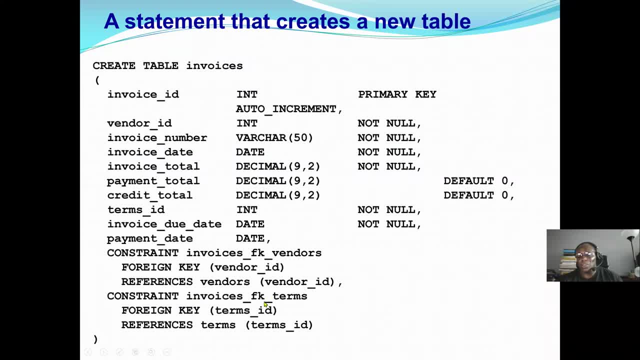 We use the same command, construct The name of the foreign key. This time we call it invoices- FK terms. The names must be unique. We can't have the same name. So this is called invoices- FK- vendors. Then we have a foreign key command. 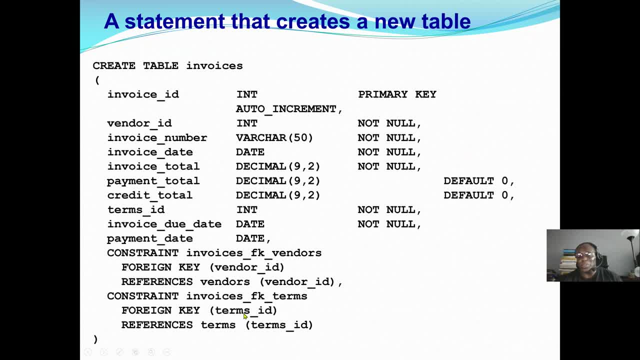 What field. Terms ID, Which means terms ID, must be a field in our invoice table, So when we look down we can see terms ID. here The data type is int And also it's not null Because it's a foreign key. 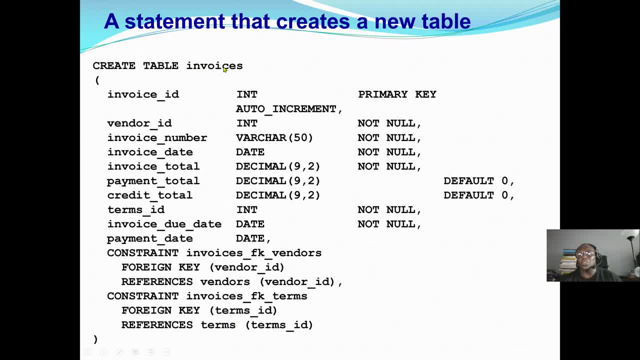 So that would be the conclusion of our first table. We have our table invoices. It has a relationship between vendors And also another relationship with terms, data and table. So we have terms table and vendors table who have a relationship with invoices. So here we see a statement. 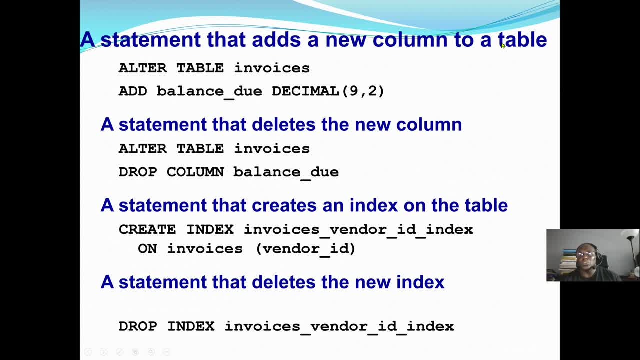 We see a statement that has a new column to a table. So we already create our table. Now we want to add a new column. Maybe we have four columns in the table. We want to update the table to add a new column, So we use the command alter table. 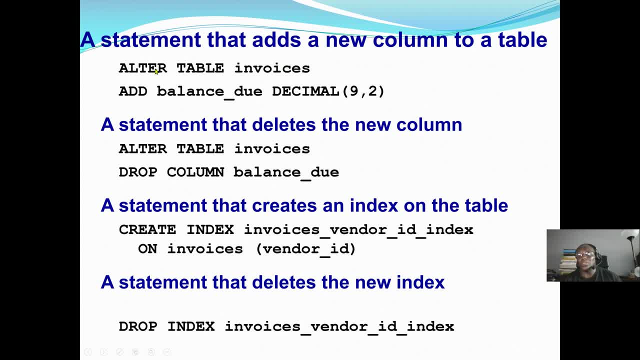 And then the table name. So this means I want to alter my table name- invoices- And I'm going to add a new column named balance deal. Balance deal data type will be decimal, with nine digits And two decimal places. So alter table command allows us to add a new column. 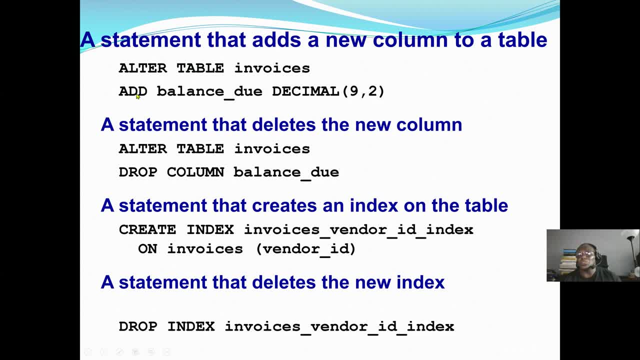 Using the hard cross. So we have alter table The name of the table, invoices, Then add command. What I'm going to add, The column name is balance deal. The column always has to have. its data type is decimal Nine digits. 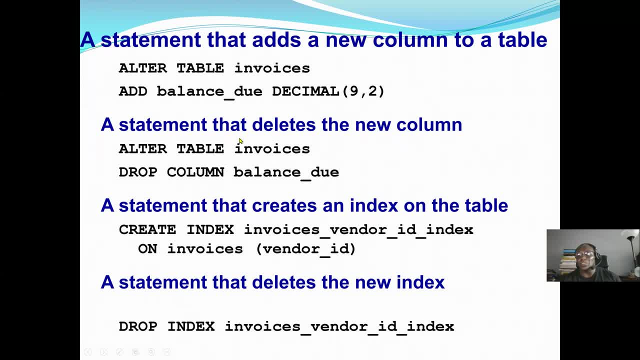 Two decimal places. Now a statement that will delete the new column. I'm still going to use the alter table And the table name, But this time I'm deleting the column, So I use the cross drop Drop column. What column are you dropped? 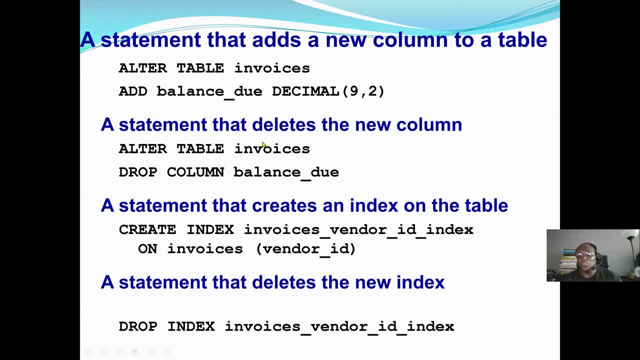 Balance deal. So alter table invoices, Then drop the column Balance deal. The first one is to add a column So hard balance deal And the data type Inverse Convert table. I use a table name. We name it vendor ID in this. 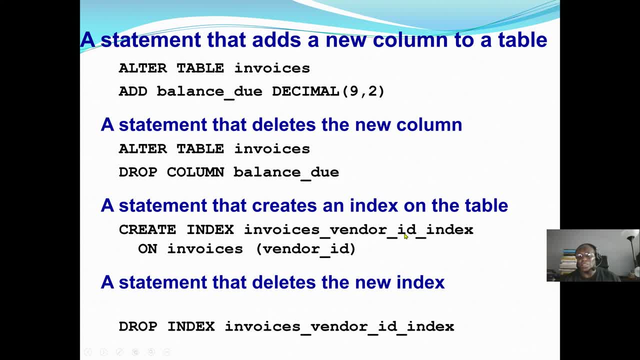 The statement that will create an index on the table. We use the command create index And the index name can be any name. here We name it invoices Vendor ID in this. Now we are creating this in this. on invoices table statement that deletes the new index, we use the command drop index and then the index name. 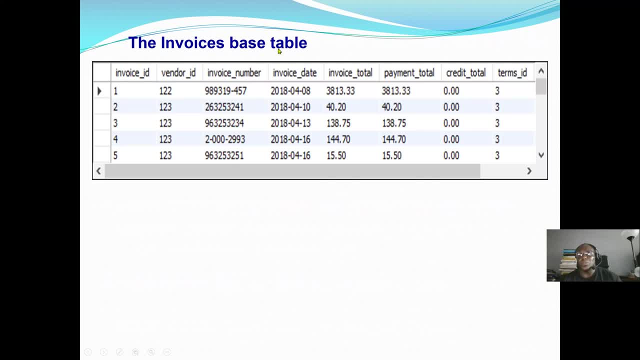 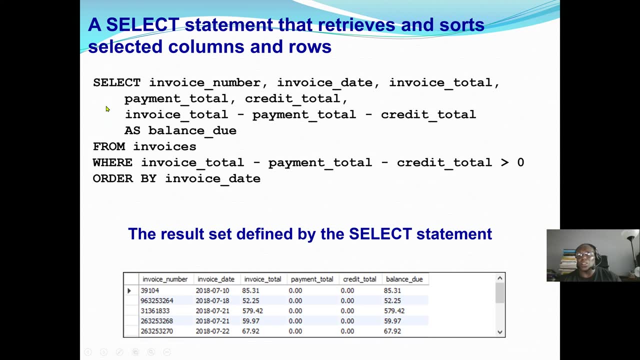 So this is an invoices-based table. We have some records Here. we want to write a query to select some items from the table. So this is a select statement that retrieves and also sorts the selected columns and rows. The select statement normally is a query. I have a thousand students in my course. I want to know all the students from. 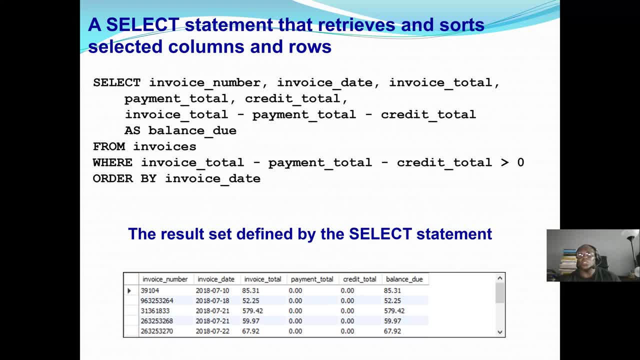 New York State or California State. So I have to write a select statement because I don't need all the students. I only need students from a specific state. So, for example, here we are dealing with invoices, I can't pay our voting. 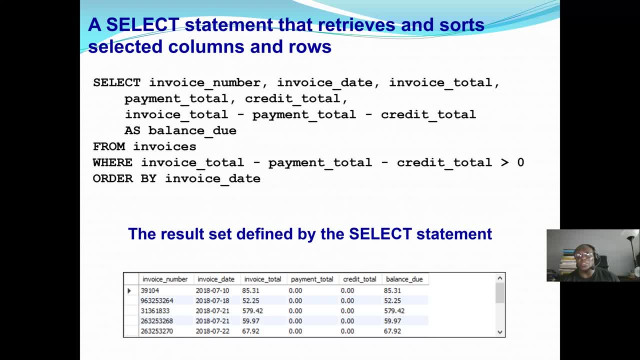 You need to set up a database system. Vendors will also apply to that. So what we are doing here is that we're going to select, and always when you start with a select statement, then next will be the column names. If you are going to select all the fields, we use asterisks. 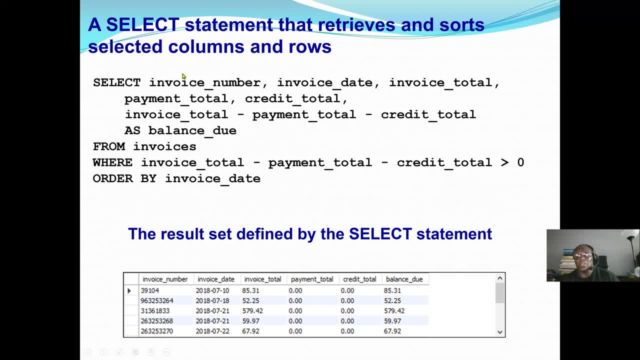 That means you are selecting all the fields in the table. But if we want- let's say we have five columns, but this time want to select only two, then we had to write the two names. But if I want to select all of them, I will have to write just one or two, And then I'm okay to write I have to. 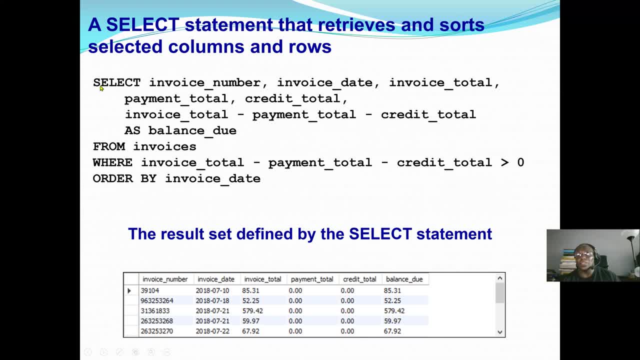 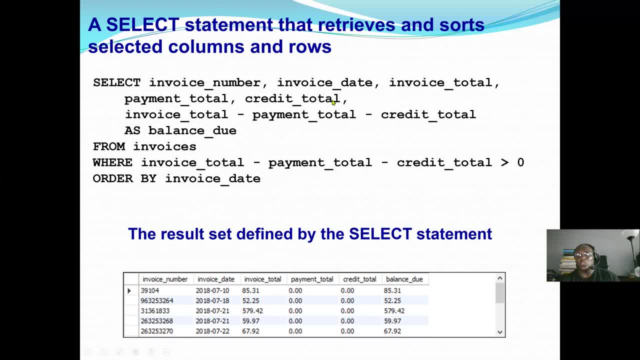 invoice total, payment total, credit total. So these are all column names and also we are going to select some item but we do some arithmetic operation on it, So we want the value which will be the balance deal. Invoice total minus payment total minus credit total. When we do these, 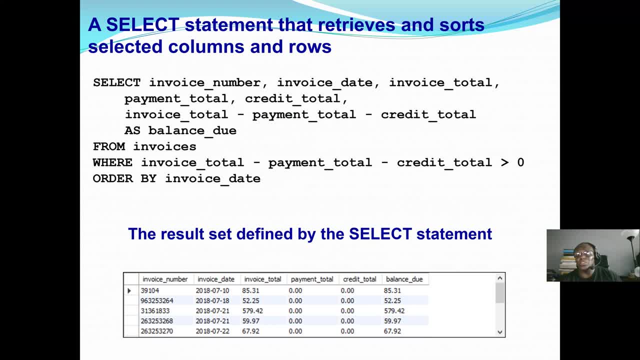 calculations. the answer we get: we put it in a new column named balance deal. So we use the keyword as balance deal. So this means I'm selecting a column, invoice number, invoice date, invoice total payment, total credit total and also invoice total minus. 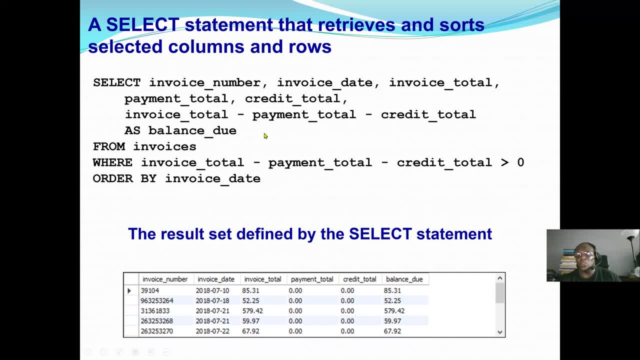 payment total. So we have all these three columns. So we do the arithmetic operation here. The answer we get, we store it in a new column named balance deal. So we use as balance deal. This information will come from invoice system, So normally select the column name from. 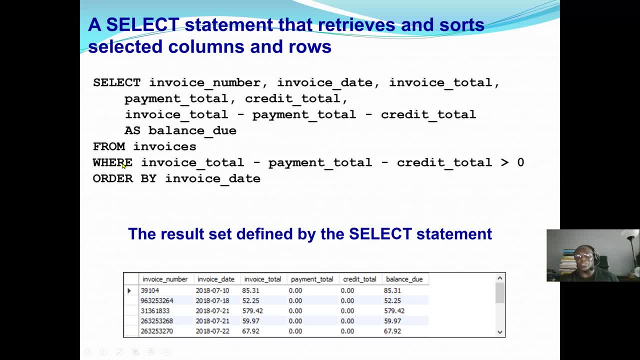 what table and also we have where. Where means the same condition. Here we have a condition: We want the balance deal to be greater than zero, which means the customer owes some money or in this case, the vendors or creditors They owe some money. So our condition says: were the invoice total. 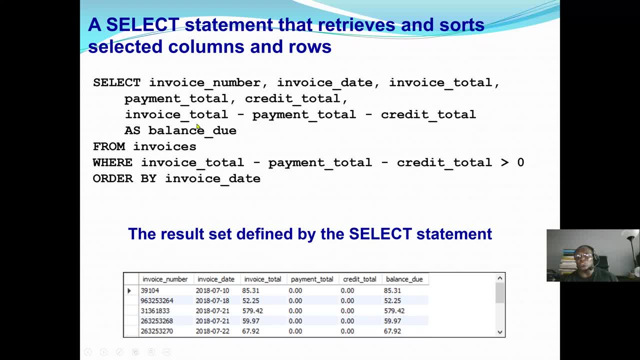 minus payment total. minus credit total- that is the balance deal formula- is greater than zero. Now, when we get the answer, we want to order it by invoice date, Which means we are going to put all the items in invoice date, Which means we are going to put all the items in invoice date. The 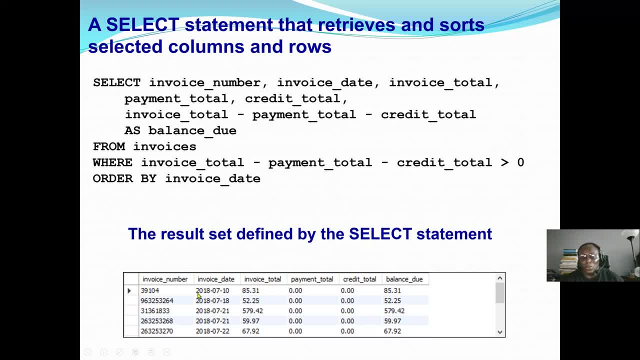 Fhazhil Wamalwae- earliest to come first. so when you look the results, you can see that we have 2018 July 10, then 2008 July 18, 2018. sorry, 2008 18, July 21, 22, etc. because we are sorting by date, so if we say order by: 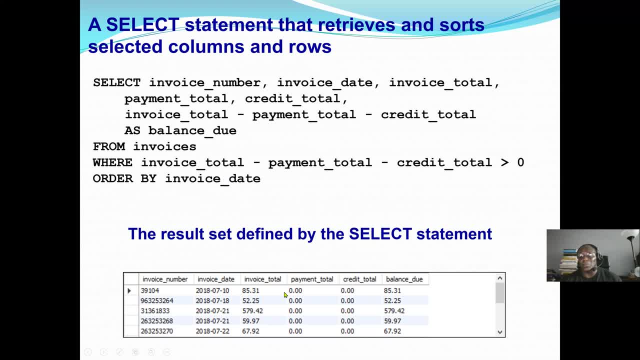 Fhazhil Wamalwae- And we didn't specify what is ascending or descending. ascending means from the earliest to know Fhazhil Wamalwae- The lowest to the highest or, in terms of date, the late to the earliest. 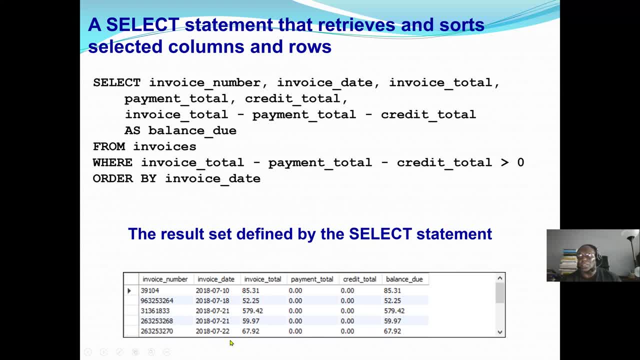 Fhazhil Wamalwae-. So we start from 10 to 22. the sending means the latest to long time ago, so we start from July 22. we go down off to July 10.. Fhazhil Wamalwae- You can see our last fit balance. do they give us the calculation for each record with the balance? is a formula we use. 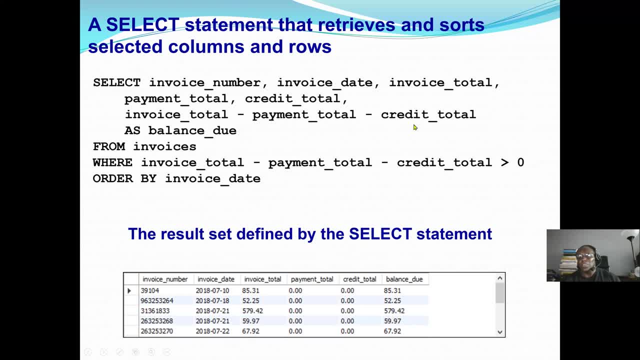 Fhazhil Wamalwae- In was still Fhazhil Wamalwae-. And then we have the word condition. so we can see that the balance do values should be at least greater than zero, or the values are positive values and not greater than zero. 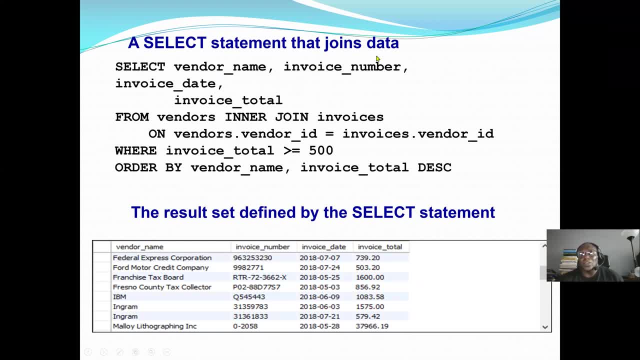 Fhazhil Wamalwae-. Now we also have a select statement that will joins data. we will go this detail somewhere around chapter four- Fhazhil Wamalwae- And SQL. we have different types of join, so, for example, you: 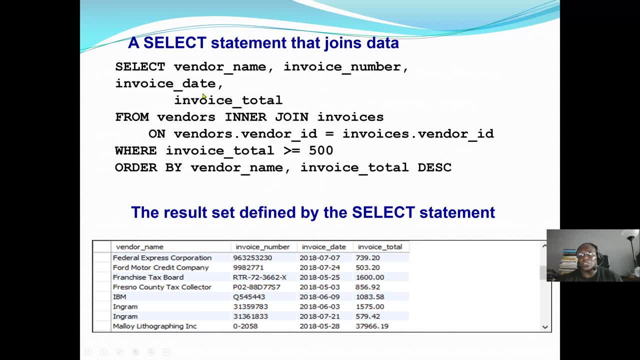 Fhazhil Wamalwae- select vendor name, invoice number, invoice date and also invoice data from vendors. in our joint invoices we use join when we want to get information from two or more tables- Fhazhil Wamalwae- Now if i'm getting information from one table then I don't need to join two tables. so here we can see that the vendor name will be in the vendors table, invoice number most likely will be in the vendors table and inverse, because he said you make fit. 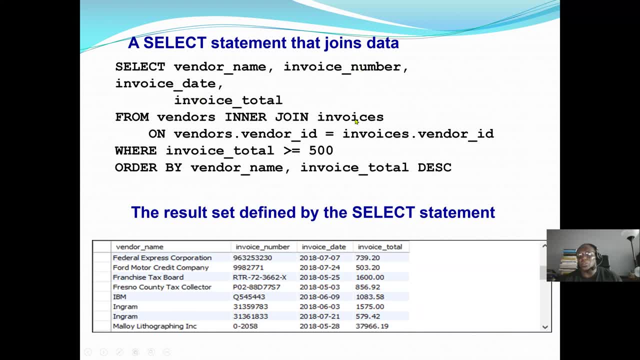 Fhazhil Wamalwae- But invoice date will be in the invoice table. so we have a vendor name in the vendors table, invoice date in the invoice table: Fhazhil Wamalwae-. So, since we are getting information from two or more tables, we created your. now, the type of job we are going to use depends on the type of data we need, the answer we need. 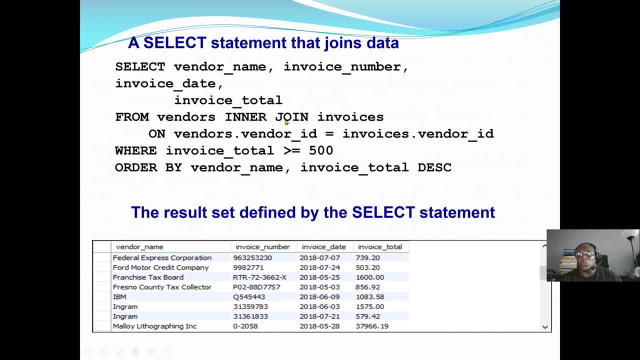 Fhazhil Wamalwae-. So yeah, we use the email join invoices and also, when we join is the same concept as you mentioned earlier- Fhazhil Wamalwae- Where we Fhazhil Wamalwae- The foreign key and the secondary key. so you can see that we are joining on vendors table with a vendor ID feed. also invoice table with a vendor's ID. 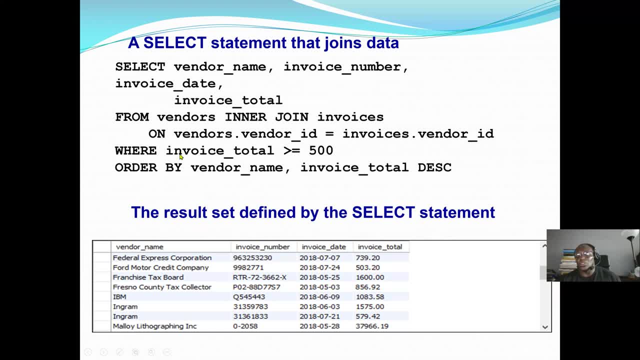 Fhazhil Wamalwae- So they must be equal. Fhazhil Wamalwae- Where he. also the invoice total should be greater than or equal to 500. so that's the condition and we are going to put this in order by vendor name and also invoiced total. here we can see, is descending the. 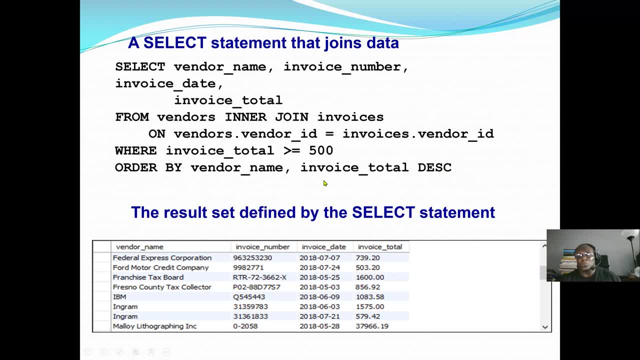 Fhazhil Wamalwae- ESC stands for descending. so when we go to the invoice total Fhazhil Wamalwae- And also the vendors, you can see that we are going to have Fhazhil Wamalwae- names. for example, if his names normally a come before B, but if it's the same, it means B will come before a. so when we look at the 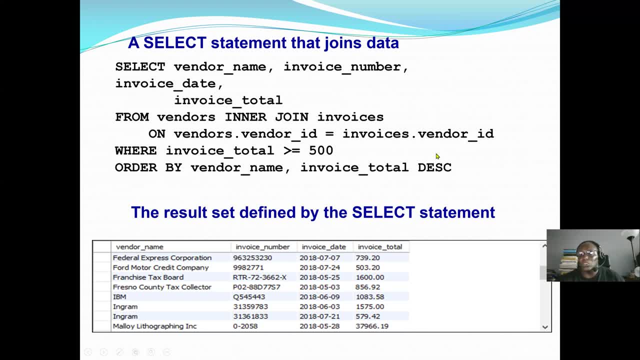 Fhazhil Wamalwae- year. we'll say order by vendor name, invoice total. so descending: Fhazhil Wamalwae- So look at the invoice total. we can see that we go from the highest to the lowest. 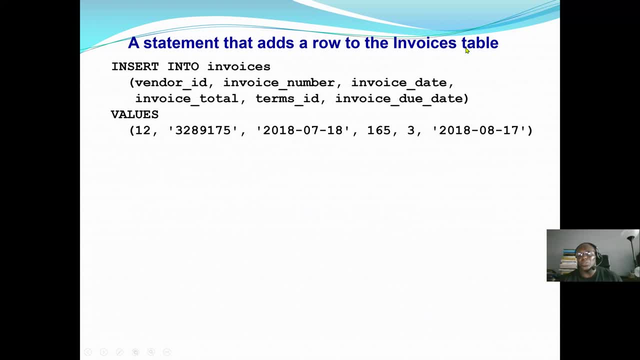 Fhazhil Wamalwae- Also. statement that will have a role to the invoice table. so we use the insert command. so the command is insert into Fhazhil Wamalwae- The table name invoices, then the fields that you are inserting to something set into vendor ID. 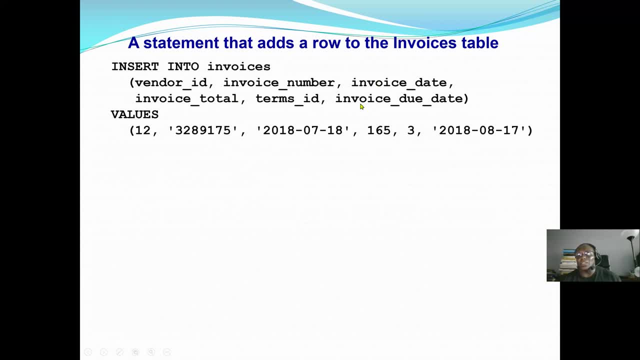 Fhazhil Wamalwae- invoice number. invoice date. invoice total: Fhazhil Wamalwae- Invoice ID. invoice due date. now the way we arrange the columns here should be the same as the values. so again, values is a command. 12 will go to vendor ID. 328-9175 will go to the invoice number, then the date to go to the invoice there. so we have to make sure that the values they are in order as the column names also. 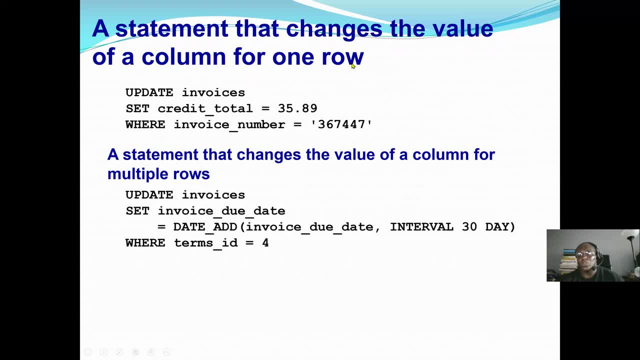 Fhazhil Wamalwae-. Now here we have a statement that will change the Fhazhil Wamalwae- Of a column for one rule. so we use the command update to change and when we say alter we are changing, for example, the column, the column in the field. but update means we are changing the record. 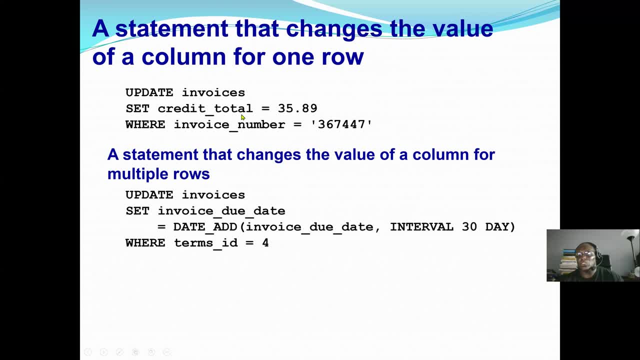 Fhazhil Wamalwae-. So here, update invoices. we set the credit total into 35.89. now, when i'm using alter, either i'm going to add more column names, i'm going to remove the column name Fhazhil Wamalwae- add or drop. 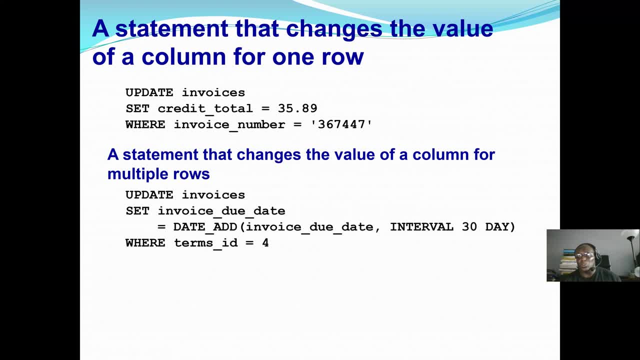 Fhazhil Wamalwae- But if I want to update a specific file, a record in the table will use the updates. come on, Fhazhil Wamalwae- So you can see. we say update. we're going to set the credit total to 35.89. 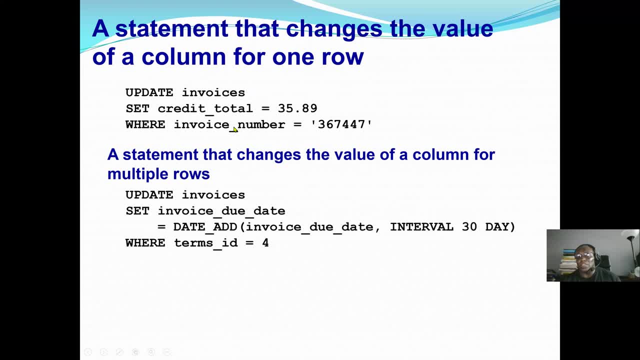 Fhazhil Wamalwae- For people or the Fhazhil Wamalwae- vendors that the invoice number is 3674447,. so if your invoice number is 367447.. Fhazhil Wamalwae- Your credit total. 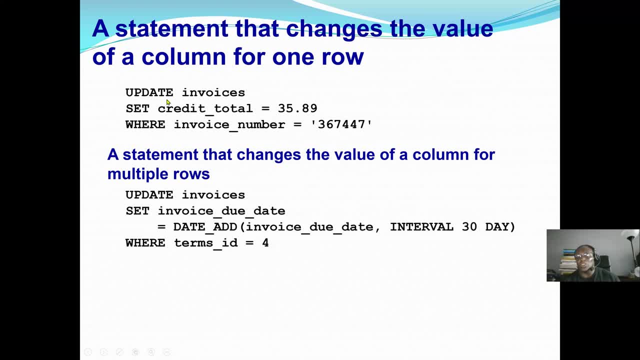 Fhazhil Wamalwae- will be $35.89. so here we say: update Fhazhil Wamalwae- The table name invoices set Fhazhil Wamalwae- credit total equal to 35.89, where the invoice number is this: 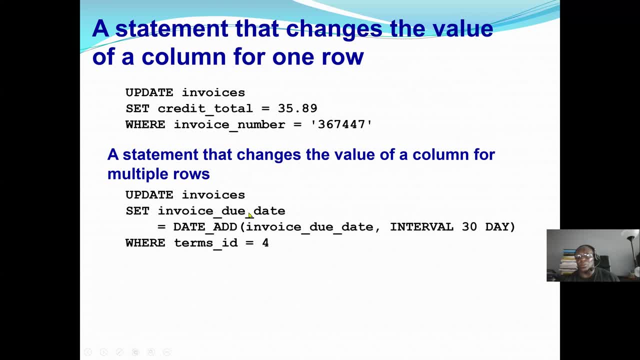 Fhazhil Wamalwae- Another example statement that changes the value of a column for multiple rows. so here we are changing the value. here is only one row- Fhazhil Wamalwae- A row that have invoice number 367447, but here is multiple row. so we say update invoices, that we are setting the invoice due date. 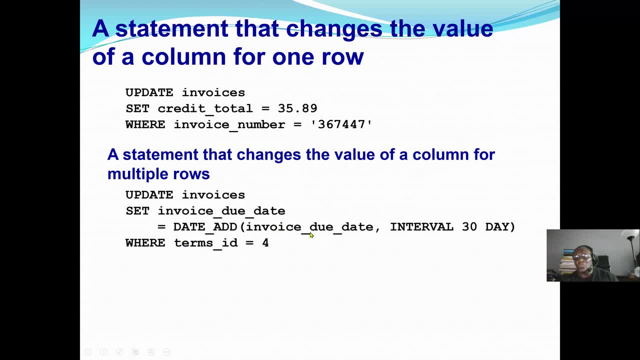 Fhazhil Wamalwae- Which equal to date, had the invoice due date interval of 30 days. Fhazhil Wamalwae- Where the terms ID equal to four. Fhazhil Wamalwae- So it's. 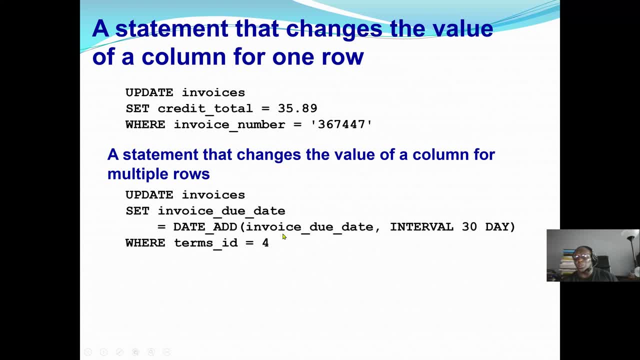 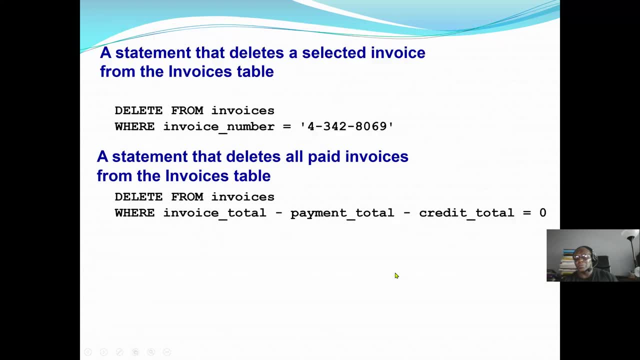 this statement will change the value of a column for multiple rows because of the condition we are being interpreted: A statement that deletes a selected invoice from the invoice table. So if I want to delete an invoice from invoice table, I use the command delete. 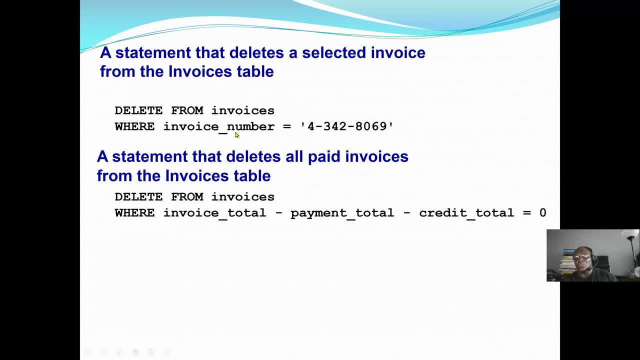 So delete from invoice the table where the invoice number equal to given. So if we see the invoice number 4-342-8069, we are going to delete it. that record Also a statement that delete all paid invoices from the invoice table. 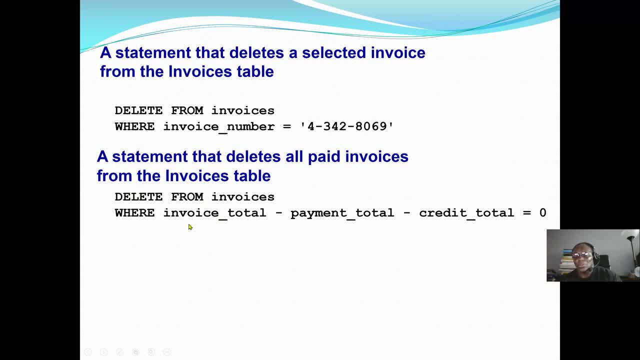 So we say: delete from invoices Because it's paid. what will happen? The invoice total, which is the bill that we have, the invoice total we have, minus the payment total, what we pay, And also minus if we have any credit before. 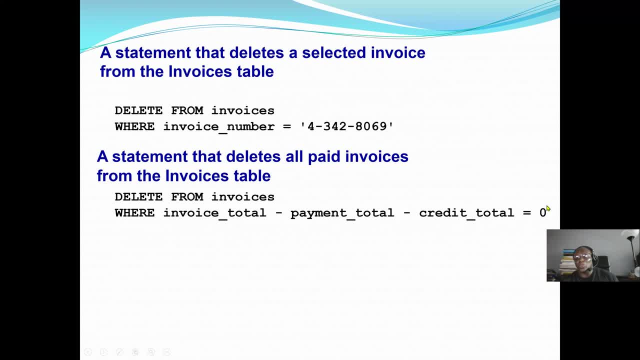 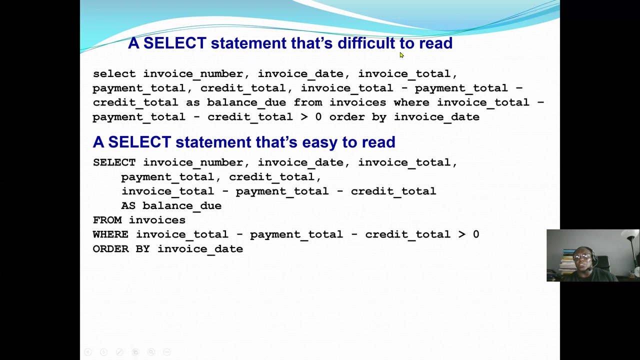 minus the credit total equal to zero, which means we have paid everything. So we're going to delete. So delete from invoices any record that the balance due is zero. Balance due will be invoice total minus payment total minus credit total. This is another select statement that is difficult to read. 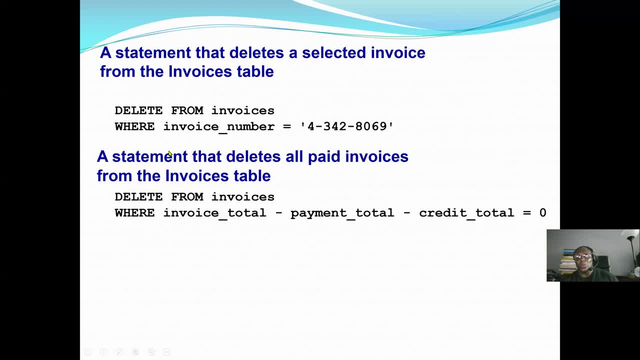 Again, as we see earlier example here, we can write all these statements in one line, but for readability and also to be very clear for us to understand is where we use the tab keys or a new line, for example, delete from invoices table. 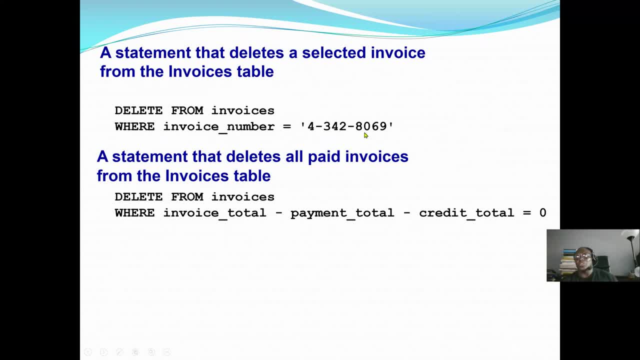 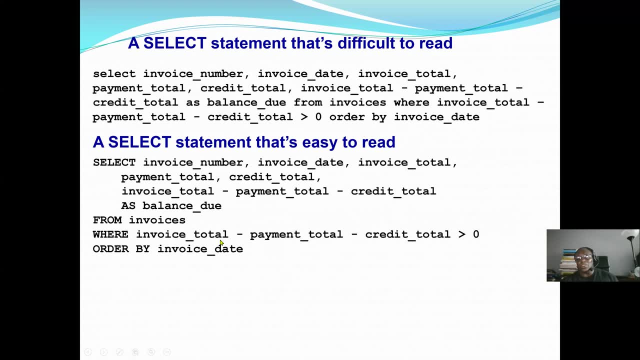 go to the second line, where invoice number equal to, instead of writing everything. So this statement is correct. It's the same as the down one, but I will prefer the down one because it's more easy to read. I can see all the columns. 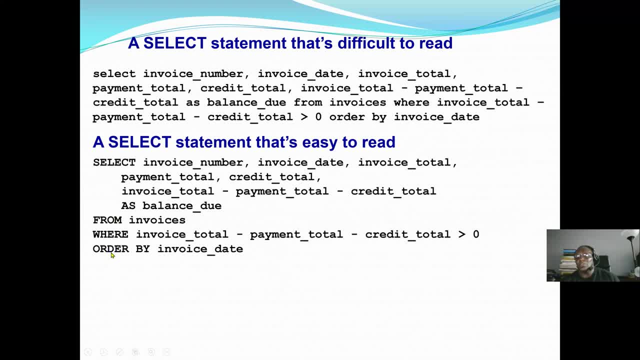 Then I can see from select from where order. I know when select come, the rest will be the column names. From the table name will follow Where there'll be a condition that we need Order by means to sort By. here we write everything. 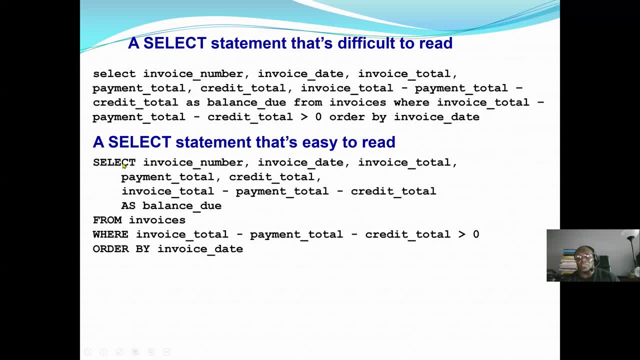 and all of them are in lower cases. You can see that here. the second is very good in a sense that more easy to read because the command are uppercase letters and the names- column names, et cetera- are lower case. 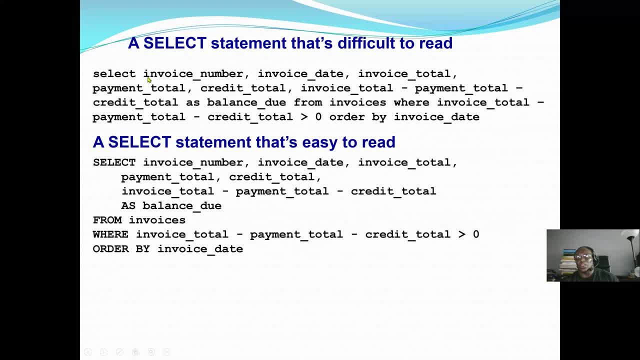 By here. everything is lower, which will be difficult to read. So select invoice number, invoice date. invoice total payment total credit total. invoice total minus payment total minus credit total as balanced you from invoices where. but you can see that everything is in lower cases. 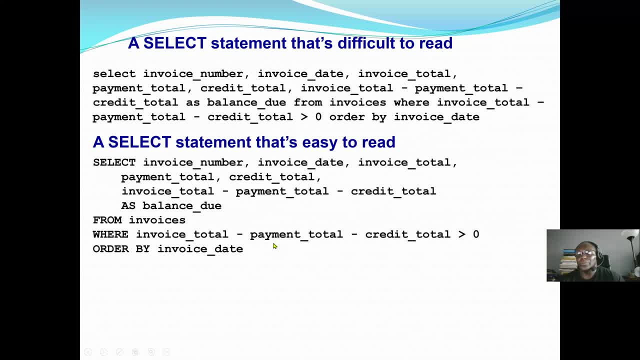 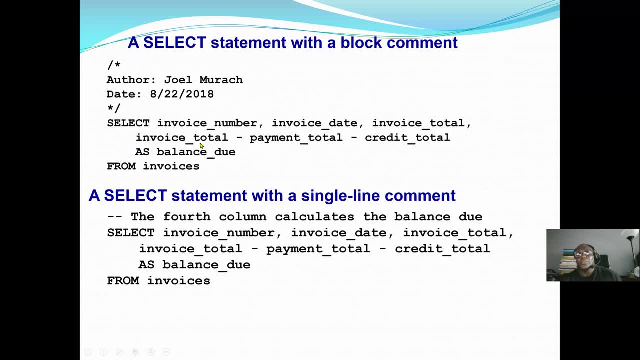 But the condition is true, So this more easy to read. select from where order? Now next also, we have a select statement with a block comment In SQL, same as Java language. we can have a comment in our statements or our file. 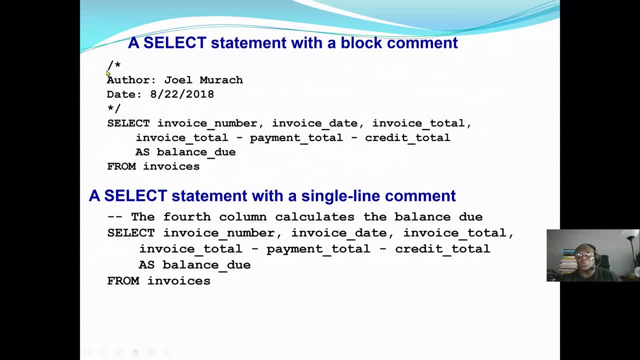 So, for example, here we have a multiple line comment. Actually, this multiple line comment sentence is the same as Java SQL, It's C++. We start with the forward slash, asterisks, Then I can write as many lines we want for comment, Then we end it with asterisks and forward slash, okay. 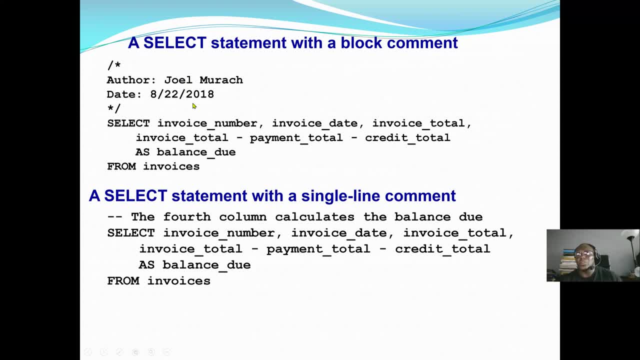 So here the comment we have is the name of the author, the person who wrote the command or the file, and the date it was written. So when we run this SQL script the comment area will be ignored by the program. So here we have select invoice number. 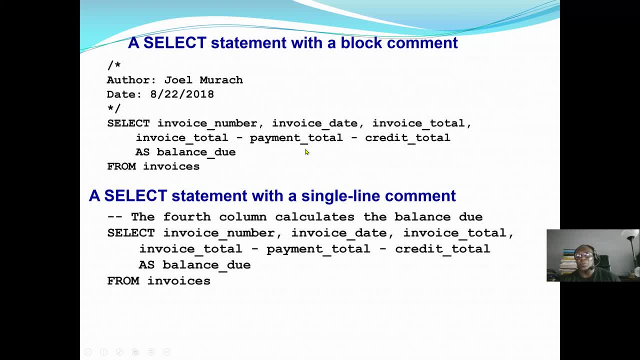 invoice date. invoice total. invoice total minus balance. total minus credit. total as balance due from invoices to. that's it Also. we may have a select statement with a single line. Normally, with single line comment we use two dashes. 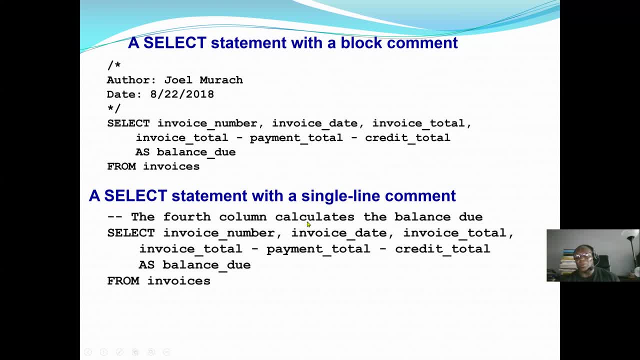 So this means only one line is the comment. the fourth command calculate the balance due. If we have more than one line, we use the multiple line comment: forward slash, asterisks. Then we end it with asterisks and forward slash- There's. yeah, we have only two lines. 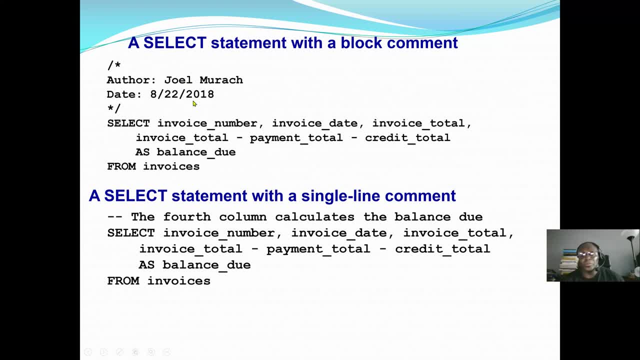 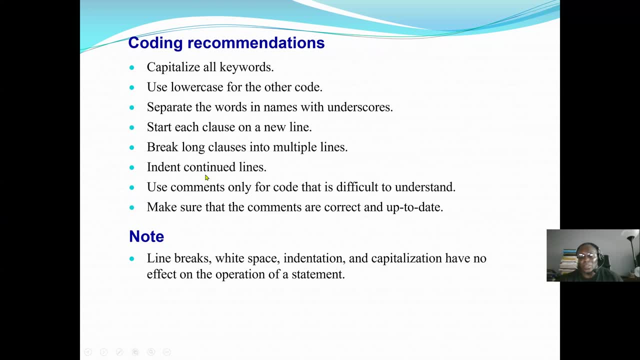 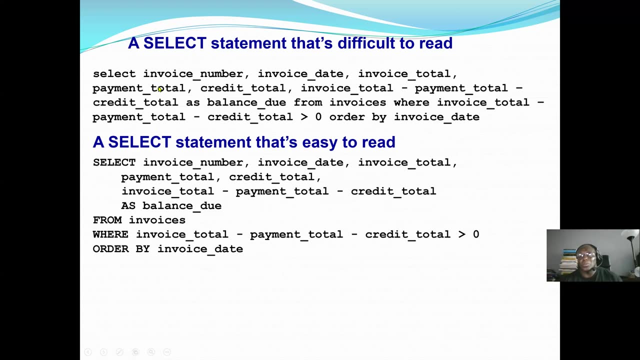 but, as we said, the lines can be as many as we want. So coding recommendation: again, we can see the previous, these two slides here we say both are the same. Again, scripts are the same, but we can see the second is more easy to write. 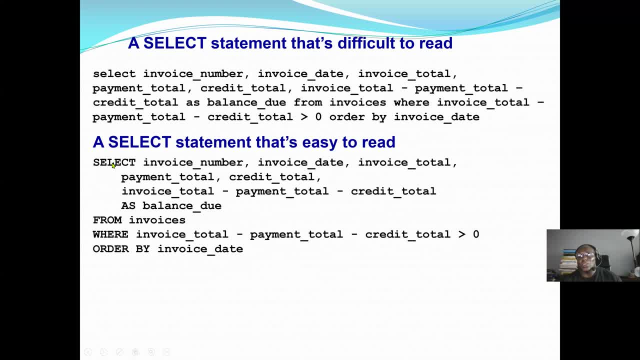 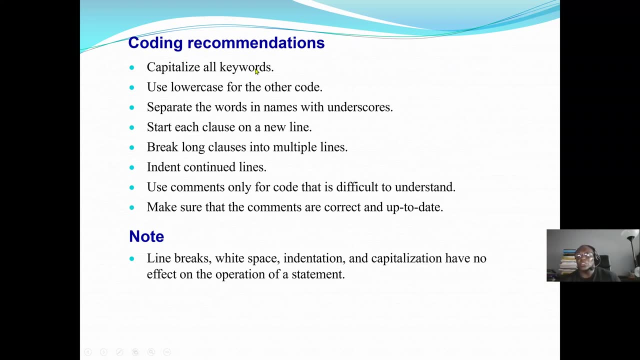 read than the first one. We make all the command upper case and the command start with a new line. I don't want to have two command in one line. So that is the suggestion here. Always we should capitalize the keywords, which would be the commands. 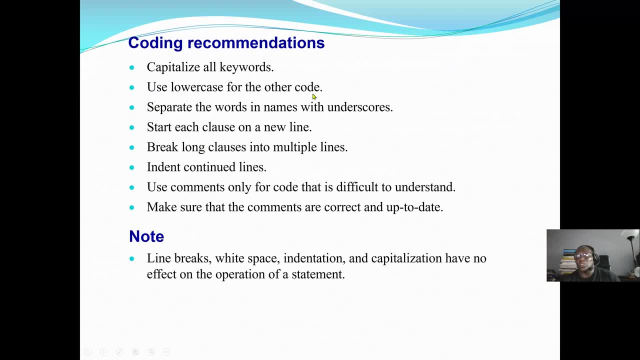 Also always we can use the lower case for other code, like the column names, the database name, the conditions, et cetera. Also we can use separate the words and names with underscores. So if I have a FK foreign key employee ID. 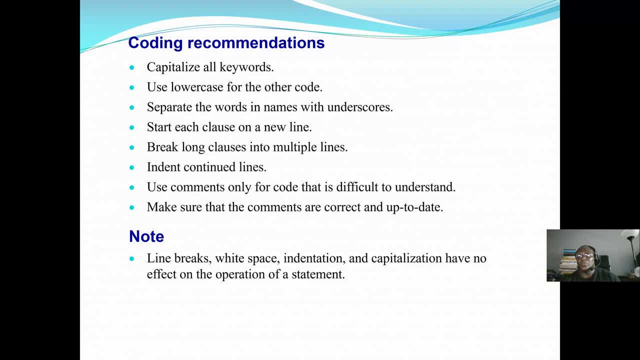 I don't want to write a space between. I will use the underscore as the space. So use underscores to separate two ways. Also, you can start each cross on a new line, and that's very good because, as you can see this example- 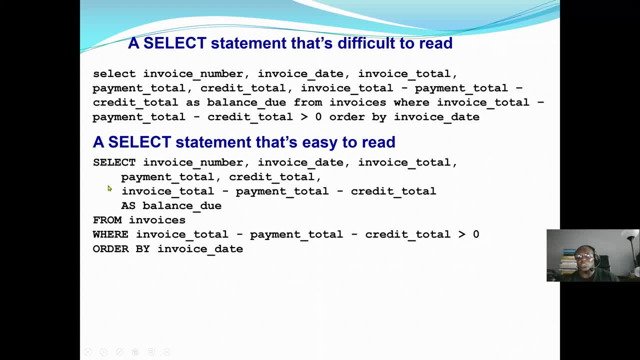 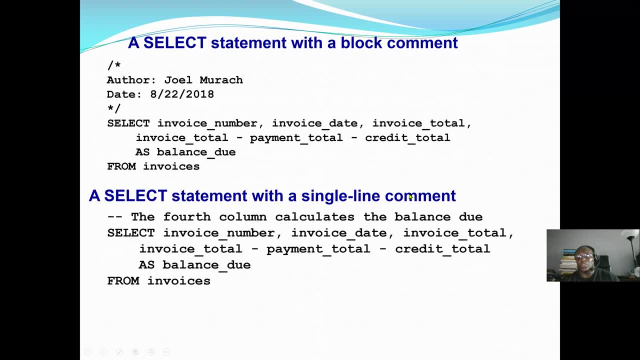 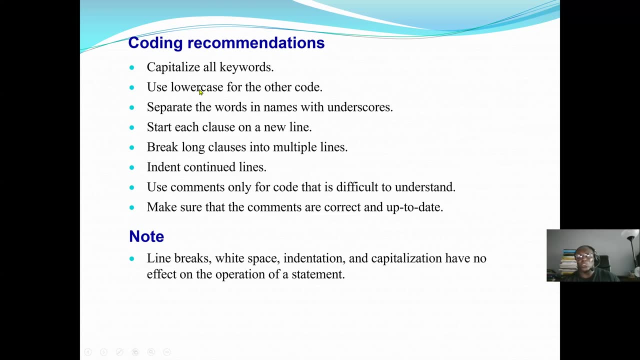 the reading was very good, So each cross start a new line. You don't want to have two commands in one line in one line, difficult to read. So again, these are just recommendations. The SQL script: we can use lowercase or uppercase. 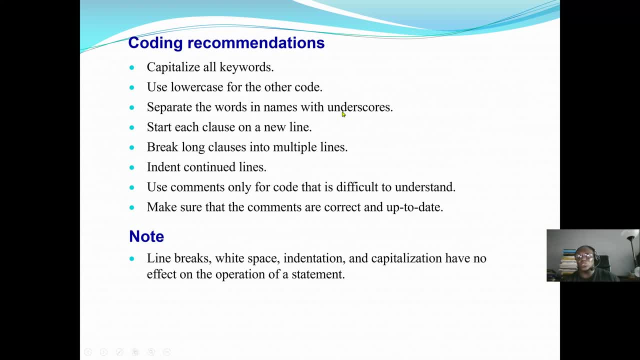 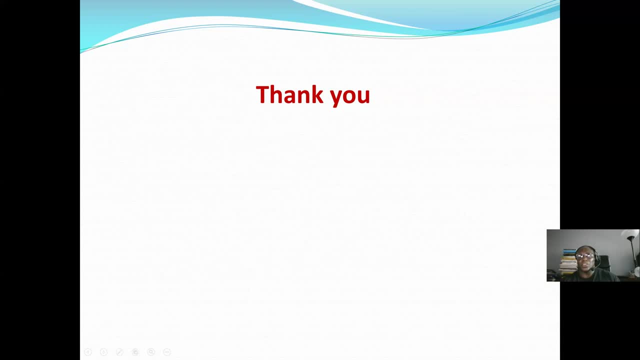 for the command. it's up to you. The names: if you like, you can use the underscores. you don't need to. it's up to you. So that would be the conclusion For our first lectures in SQL. Again, this course we are using MySQL database as our lab. 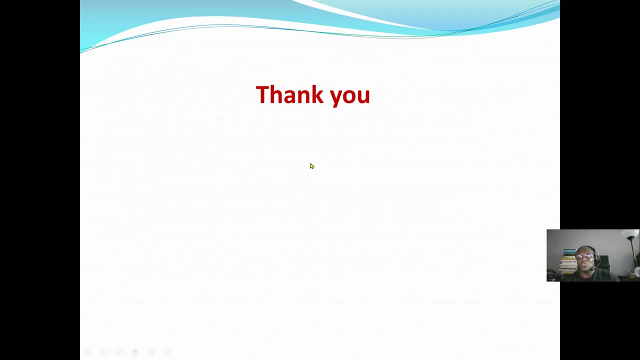 So all the commands we have here will 100% run on MySQL. In our next lectures we're going to study how again to use my workbench and also how to download it. So again, wish everybody the best, Thank you. Bye-bye.